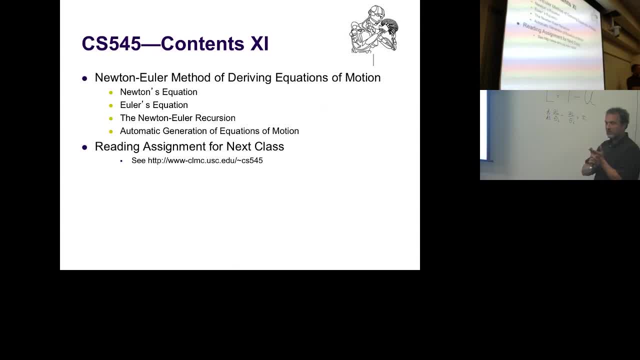 Linear or translatory energy and to a rotational energy Potential. energies always involve gravity- pretty straightforward, and the main component which we needed was our knowledge of kinematics so that we could go to the individual points on the robot, figure out where they are, where the center of mass is and things like that. 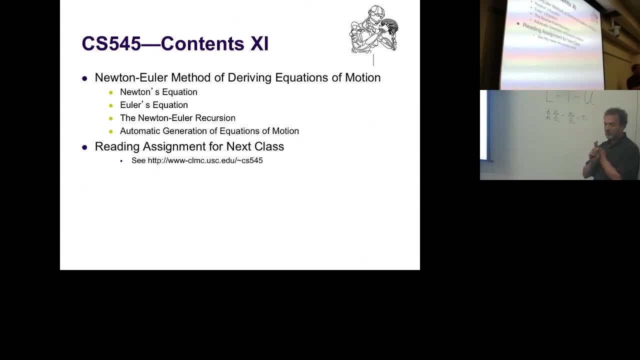 and also, what is the velocity of a particular thing which we get from Jacobians? We do know how to handle Jacobians. All of you can answer all of you which is yes, and why is it not looking like that? 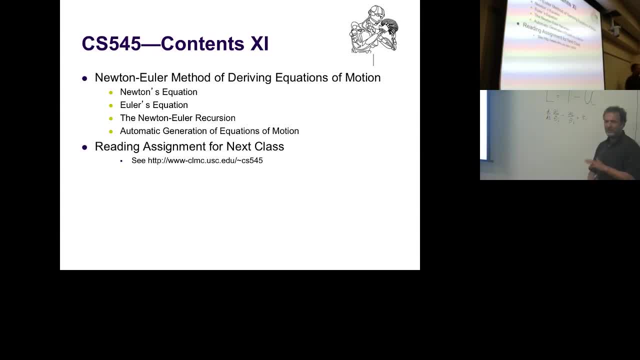 Anyway, I assume you know the Jacobians, so we'll bother you most likely in a moment with Jacobians, just to make sure that you know them Good, This differentiation is lovely, but it creates an enormous amount of terms if you have a. 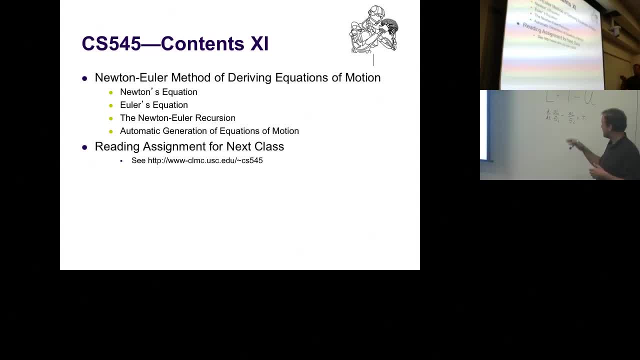 complex robot. It basically fills pages and pages literally. I ran this a long time ago For a 70-degree robot arm, like my arm through Mathematica, which is this symbolic manipulation system where you put everything symbolically in there and then you do differentiation. 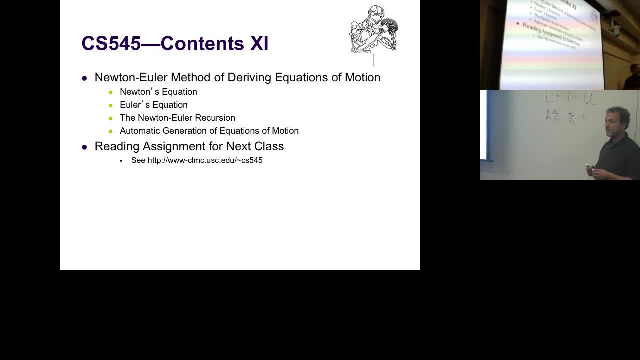 and then you have afterwards like literally three, four hundred pages of code at a time. It's totally inefficient. For that reason people were thinking really hard how to make it more efficient and there is something very simple which kind of indicates there might be something which is more efficient. 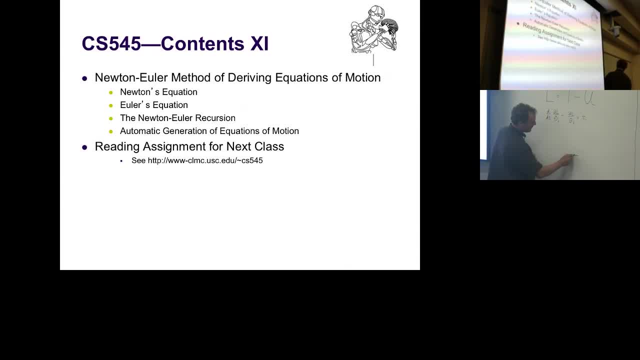 Most of the time it's not. It's not So for most robots, particularly those which we come to look at. they are open chains. They may be branching at some point in their fingers, their ears, So there's a simple way of going through that. 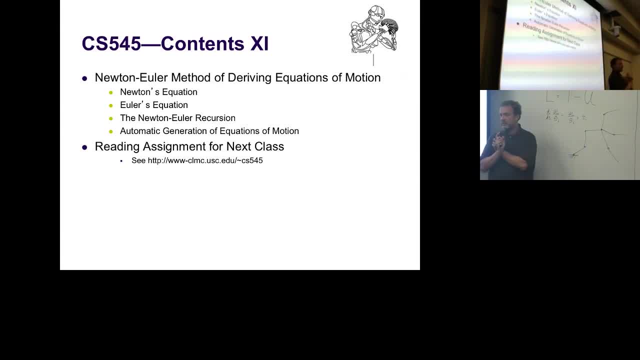 It's already what we've been doing with homogeneous transformation matrices for modeling direct kinematics: One degree, next one, next one, branching out, branching out, branching out. So there's a sequence. When there's a sequence, there's usually a potential for recursions. 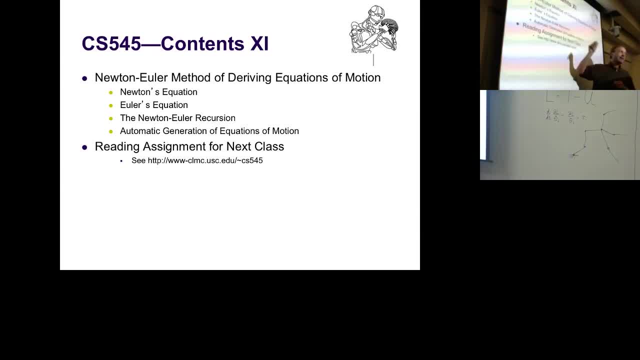 And that's essentially what Newton-Euler is about. It basically tries to go in a different way. It looks at what is called force and momentum balances at every link and then tries to relate unknown quantities to the previous link or to the next link. 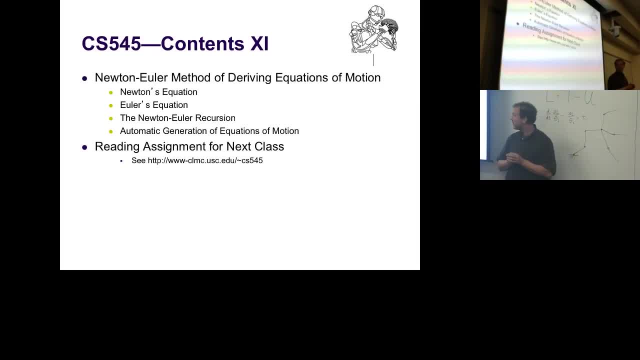 And that creates a recursion which makes everything much, much simpler. So in the end it turns out that Newton-Euler equations for my seven degrees of freedom arm just become like whatever. five, six pages of C code rather than three, four hundred. 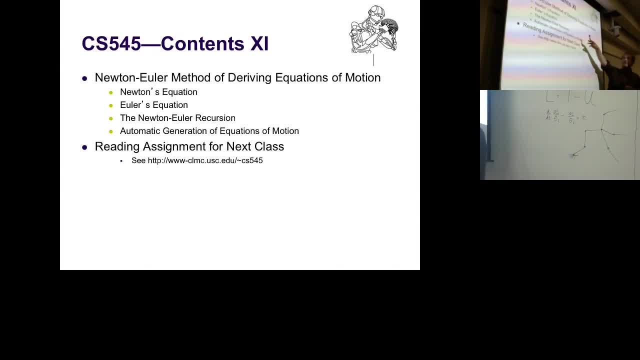 And that is a huge difference. So Newton-Euler, the real good versions of it. they are solidly linear. Basically, the computation which you have to do is linear in the degrees of freedom. But this is from a computer standpoint. it's quite nice. 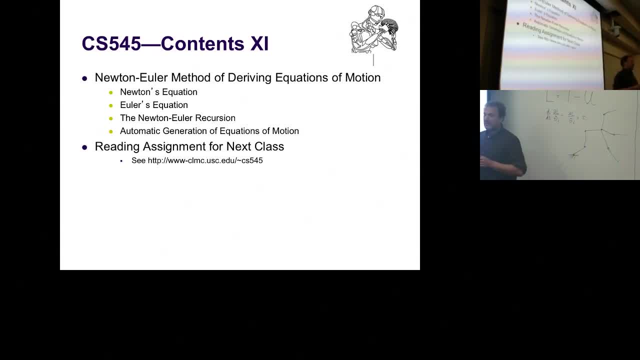 So because this is used a lot and because there's a lot of useful physics in that, our technology is trying to run you through this one time, It's painful for me a little bit too, since there's a lot of notation which goes into that. 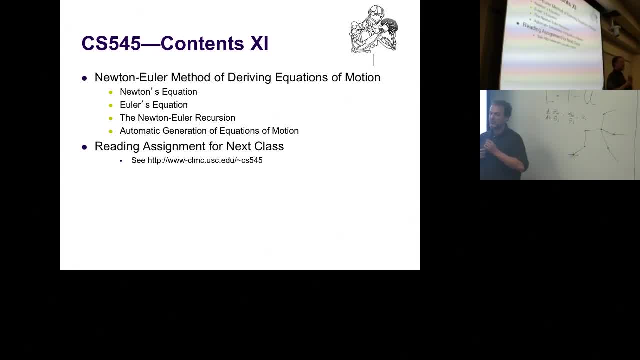 In the end you will not be quizzed on that. in terms of that, you write Newton-Euler for me and the quiz is not going to happen, But it's good to know about it. You know I had this very fun experience once in this course, after the fourth lecture. 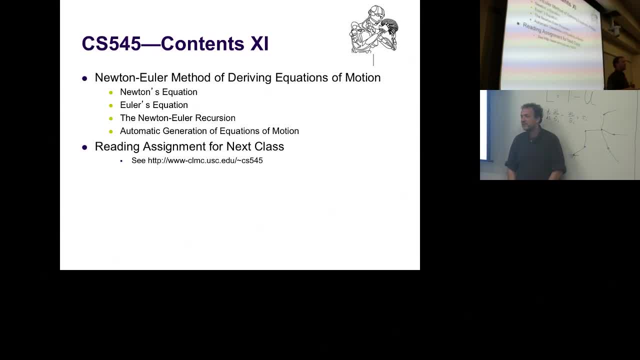 and someone said in the background: it's all about physics this course- Yeah, it's all about physics. Robotics is about creating forces and torques to manipulate forces, To manipulate bodies to do something you want them to do, And that is, by definition, physics. 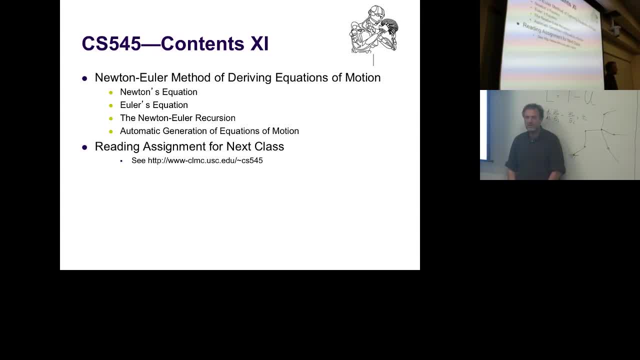 And without a physical intuition, you will never understand a robot properly. You need to simply see that there's forces and torques and how they act and what they do, And you need to get your high school physics out and maybe a little bit of your whatever. 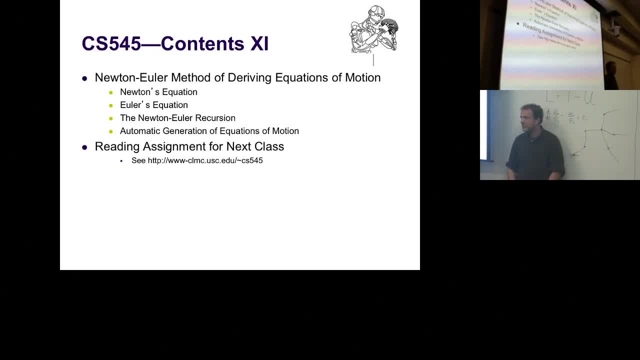 college degree physics and feel the force. Luke, they eat forces And they are dark forces and good forces. And good forces push you where you want to go. The dark ones make you fall over. So it's all there, you know. 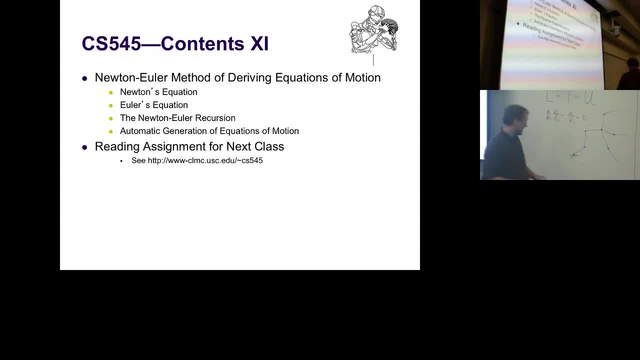 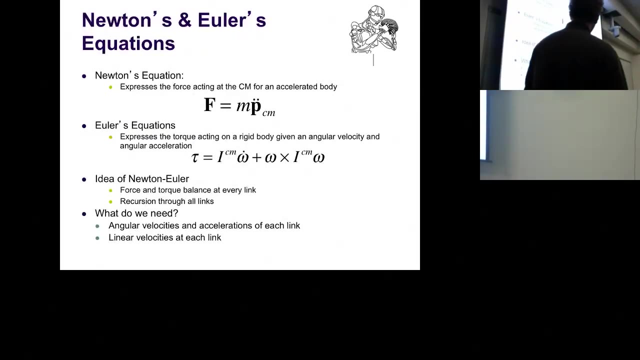 Star Wars. they all anticipated it. Good. So let's go through that, As painful as it may be, And I may goof- okay, This is something which I always have to get going myself- But here is what we start with, and that's actually not so bad. 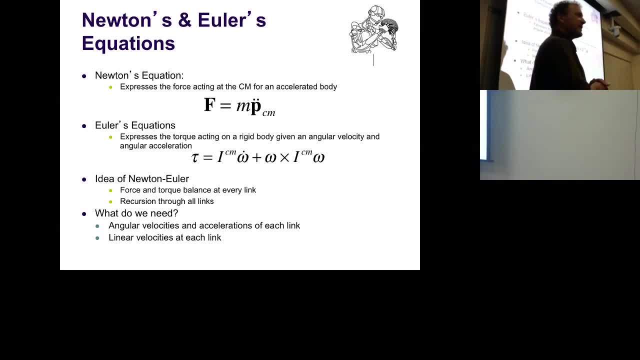 Newton. once upon a time, It was about 500 years ago- There was a guy who was watching apples- Not really. This seems to be total BS, But anyway. stuff falls And basically the idea is: a force comes from a mass which is accelerated. 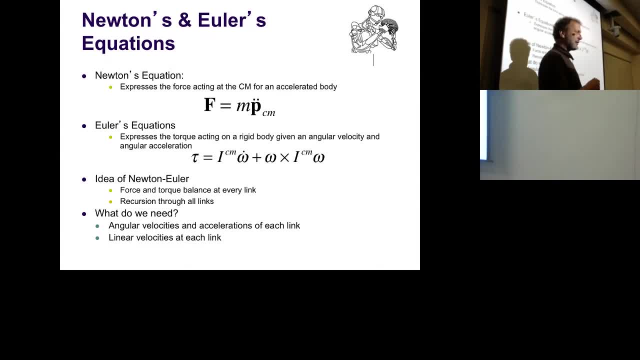 Mass times, acceleration, Mass times, gravity is our gravity force. okay, One of the fundamental laws which holds quite nicely here on Earth. If you want to go up and do things at the speed of light, things change. But that happens to very few of us. 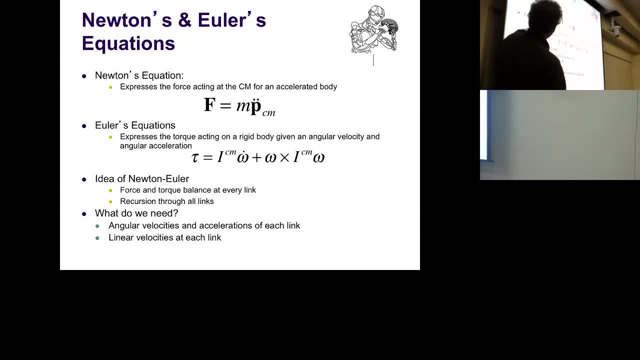 So Newton's equation, And then there is an equivalent to Newton, which is Euler's equation, which just basically makes the same statement about torques. So whenever you basically have a rotating body and you try to change its way of rotating, you need a torque to do that. 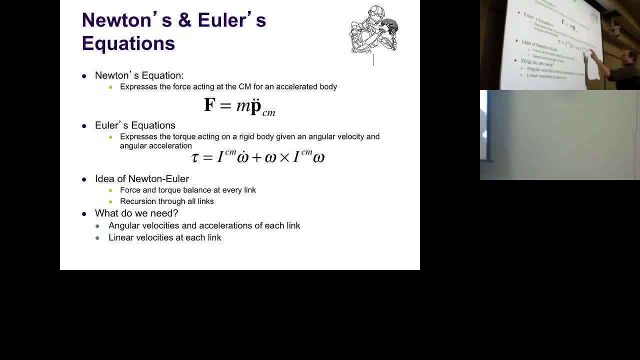 You know, what is the most beautiful example of life about these kind of Euler equations? Euler's equation is bicycling. okay, Bicycling is basically the balancing torques, because your wheels are big and they rotate. And guess what? They don't want to fall over at all. 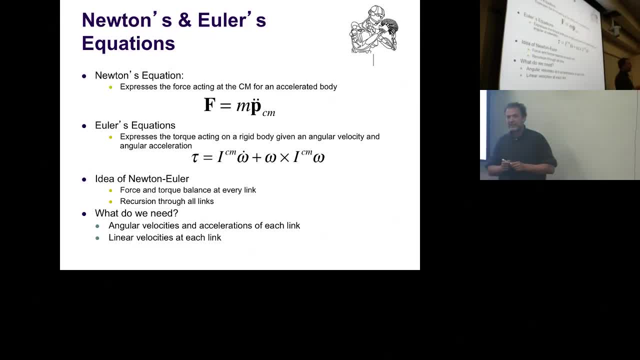 It's just a stupid driver on top who wants to fall over. And all that you need to learn on your bike is just learn how to deal with a physical system which, by itself, wants to balance. And if you don't believe me, here's an experiment for the night. 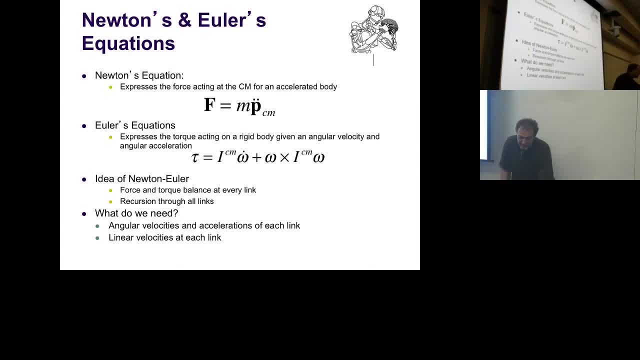 You go on a hill, You take your bicycle, Give it a push downhill And see how far it goes. See how far it gets, And you'll figure out it goes quite far before it falls over. It just tells you your bike is actually capable of biking without you, which is very cool. 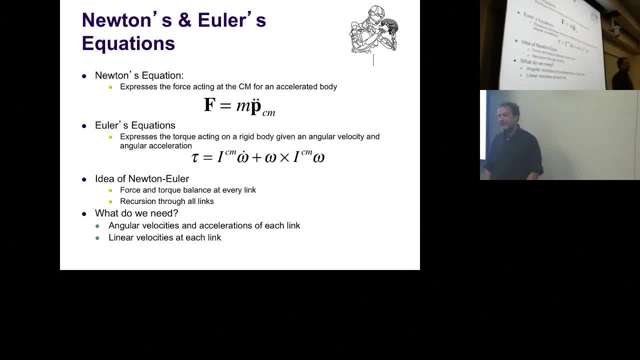 And that's essentially what this equation kind of encapsulates. It says you can only make this thing go away from its direction of rotation by applying forces And by default it actually wants to not get these forces applied. If you want to fall over, you have to apply a force. 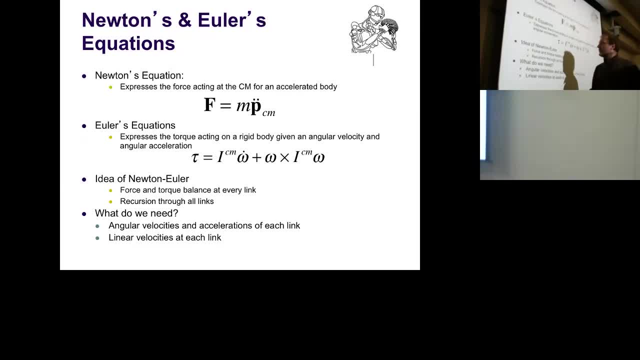 It's not happening by itself. OK, So then the idea of Newton Euler is essentially a force of torque balance at every link in a recursion through all links. Before we get to the beauty of physics, we have to do something really annoying. We have to first figure out something which is angular velocities and angular acceleration. 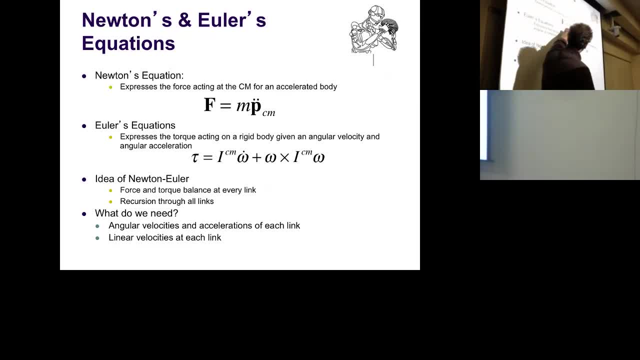 at every link and linear velocities at every link. So we look at those equations. What I'm going to do in the end is I give you some whatever link body again, which I don't know how to draw very nicely, But something like this: 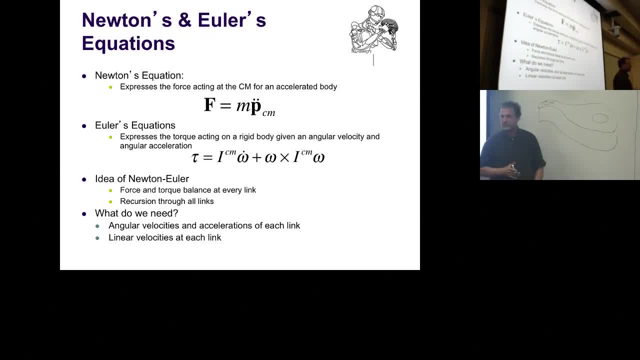 OK, And I want to basically argue about all the forces and torques which are here, But in order to compute them and to relate them to the mass and inertia of that link, I need these quantities: I need P double dot, I need omega dot and omega. 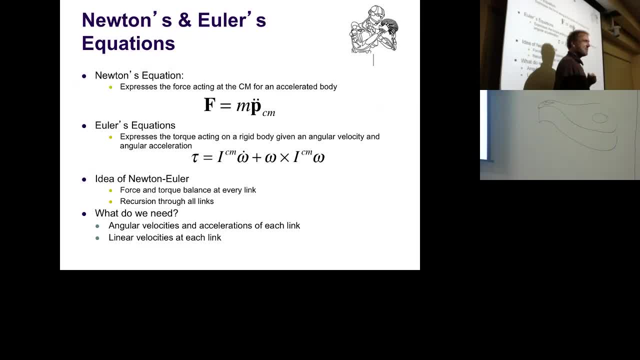 Now omega, we know how to get. You're good at this. This comes from the Jacobian, remember? We did this the last time for kinetic energy, P double dot. we haven't really cared about yet, And omega dot is just the angular acceleration. 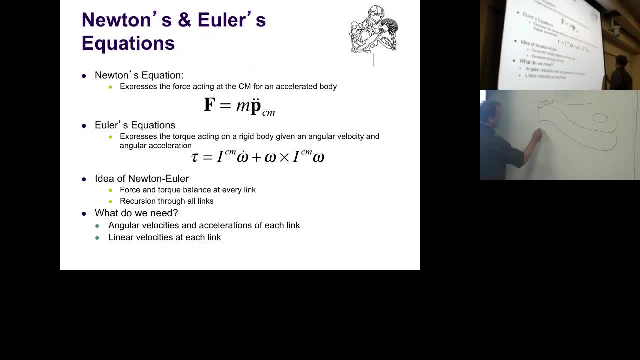 Or it would be. if we wanted to write it in joint angles, it would be the double dot, the acceleration. We'll talk about that. We'll see how it relates to that That. we don't know how to do yet, So we have to do a tiny little detour and talk about this first, before we do this nonsense. 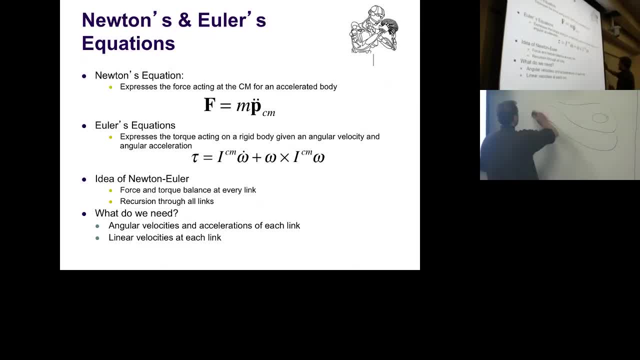 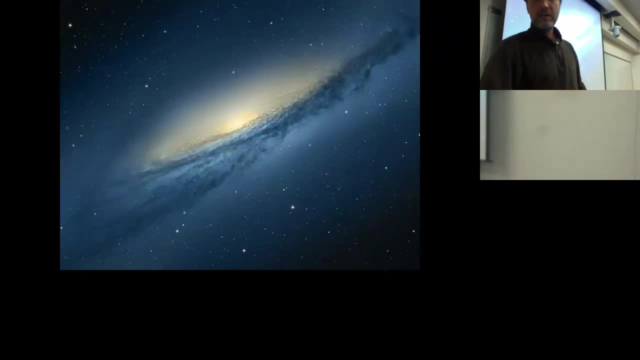 Not now, Absolutely OK. The book has two chapters. on that, I'll just hop back to the book for the moment. I'll try to explain that as much as I can. And it all starts with this: The window is still too big. 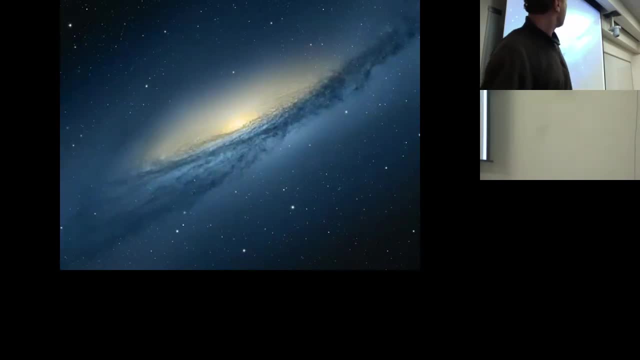 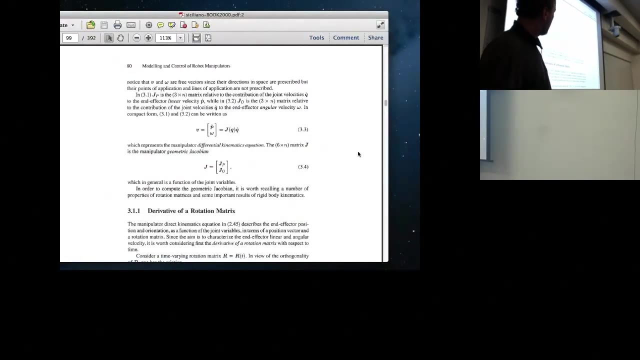 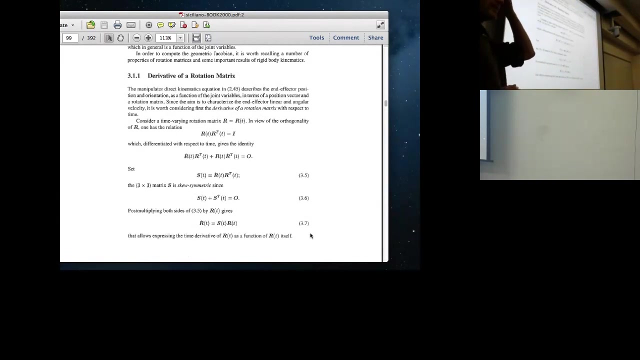 Sorry, Working on it, Here we go Now. it should be fine. So this is actually. at the end of the chapter of forward kinematics comes a quite cute little chapter about the derivative of a rotation matrix. So why do I care about this? 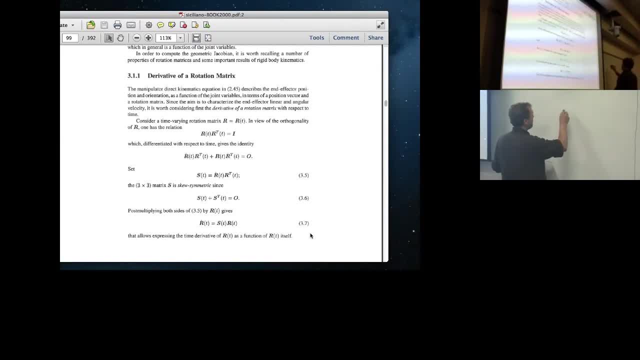 Because, remember that we've expressed a point, If I have my favorite potato body which is out here and there is a particular point of interest on this potato body, which I call now p, expressed in coordinate system 1.. And then here is the main coordinate system. 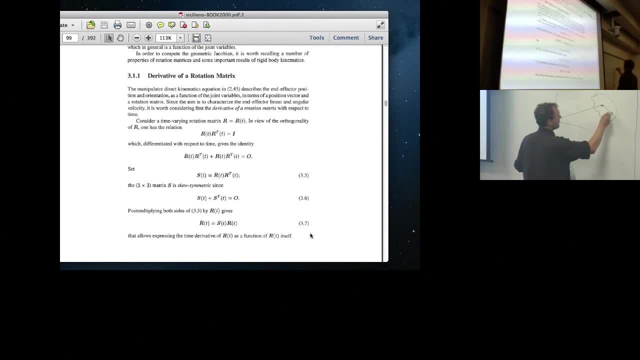 And I want to express this point here- For the offset vector, which you can call O, from 1 to 0.. This is usually what The vector r in, 1.. And then this here is the vector p, expressed in coordinate system: 0.. 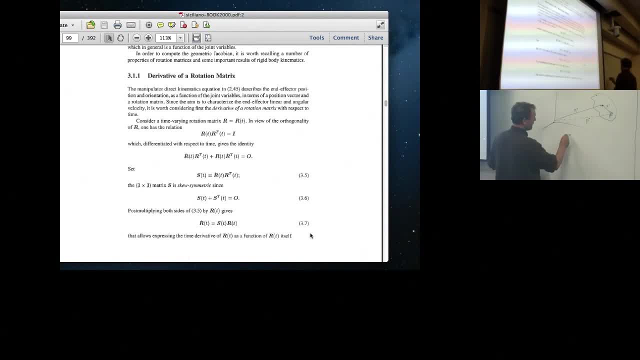 So we have essentially that p in 0 is usually something like O, the offset vector, plus the good old transfer rotation matrix from 0 to 1 times p 1.. OK, Makes sense. Now I want to get to linear accelerations and angular accelerations. 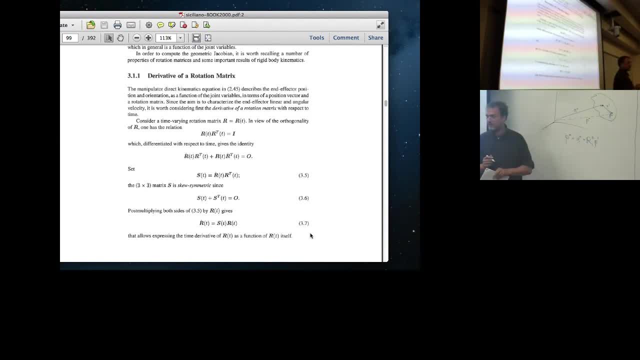 It means I have to put somewhere dots, And ideally I would just put two dots here, two dots there, two dots there, and that would be good. It's totally wrong. So that's not going to fly, Because the rotation matrix is also a coordinate system. 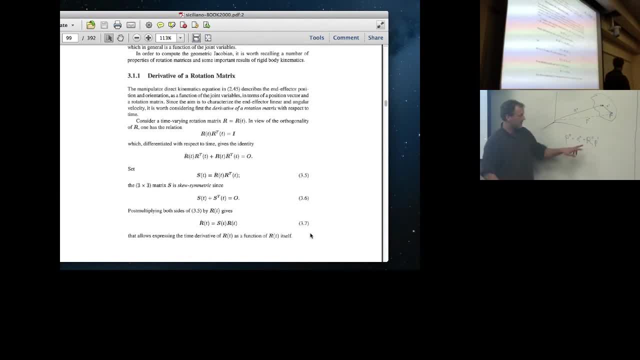 It's actually which changes with time. So what's the derivative of a rotation matrix is the question of the day. That's essentially what this chapter addresses And it's actually really cute. It's a little annoying And maybe it's not worthwhile deriving. 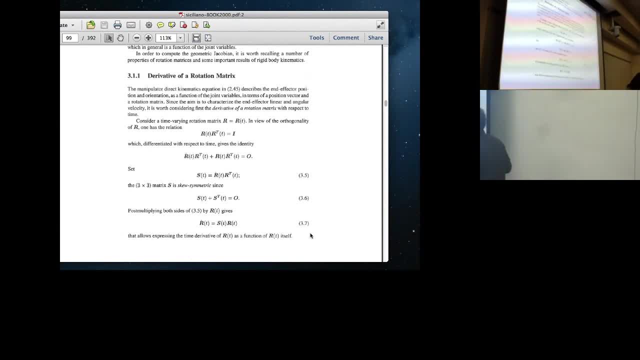 But actually it has a useful insight, And so that's why I want to go through it. So we started with something which is based on any rotation matrix times. its transpose is identity. OK, Do you agree with that? Everybody who does not agree just get out of here. 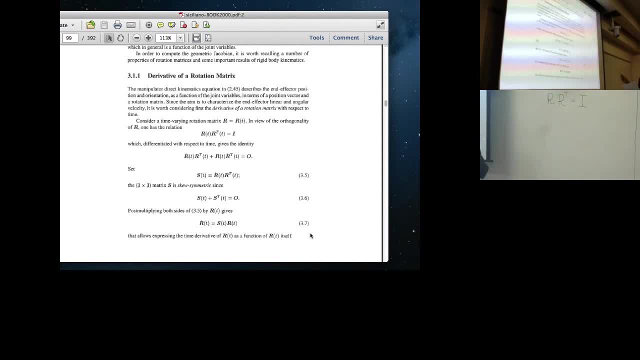 OK, Lots of people are not here, Maybe they don't. So next thing is we take the time derivative of that. So that's actually not too hard. So we do r dot times the chain rule, So that's mr times r dot transpose and the time derivative of the identity matrix. 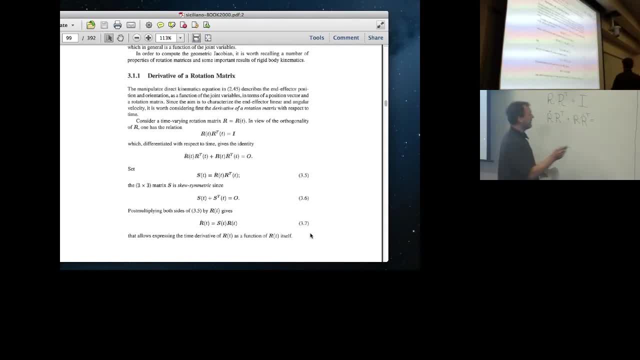 So what's the difference? Yeehaw, It's a change, It's a lovely time. derivative, It's just zero. So hopefully I created this thing here And now he basically makes a substitution. So he substitutes r, dot times r. 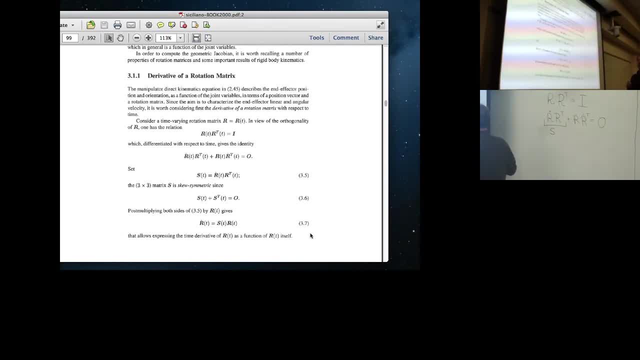 He calls it s OK. And then this here is essentially s transpose, And given that s Plus s transpose equals zero, It must be a skew-symmetric matrix. We learned that in the linear algebra I started. OK, Fine, This just tells a little bit what this thing looks like. 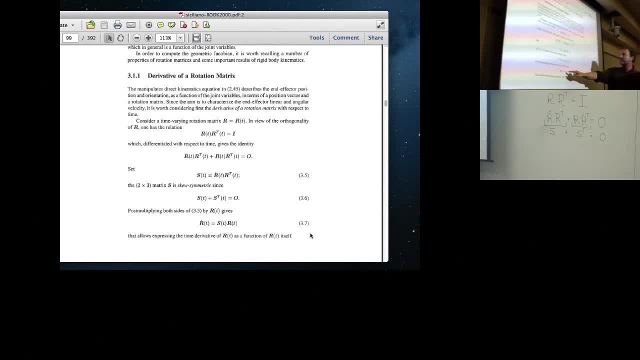 Now what does he do next? So basically, he puts this equation here. What does he do? Da, da, da, da, da. Post-multiple sets: Post-multiple sets of 3.5.. OK, Go Now to the s equation. 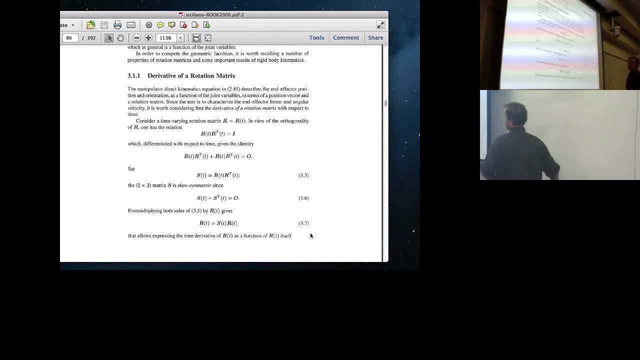 It's kind of a weird little derivation. So we take this equation s equals r dot times r, transpose That is 3.5.. Post-multiply both sides of 3.5 with r of t. So basically we multiply it with r. 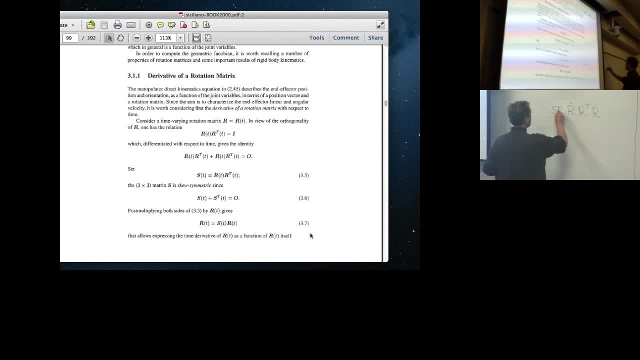 And also with r here. OK, You get this. And then he basically says This. basically says This: here becomes identity. So r dot equals s times r Interesting. So that tells us something about how to express r dot in terms of r. 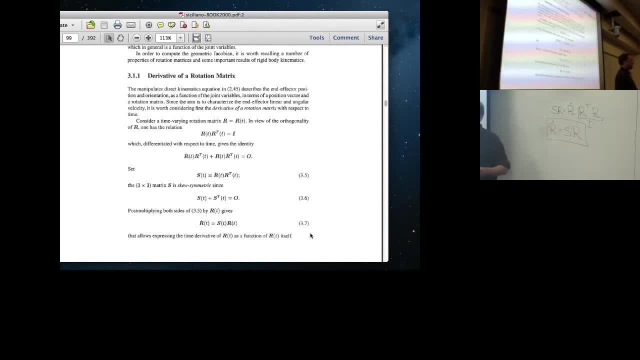 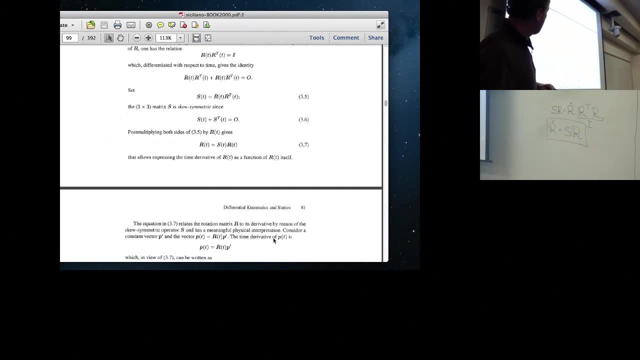 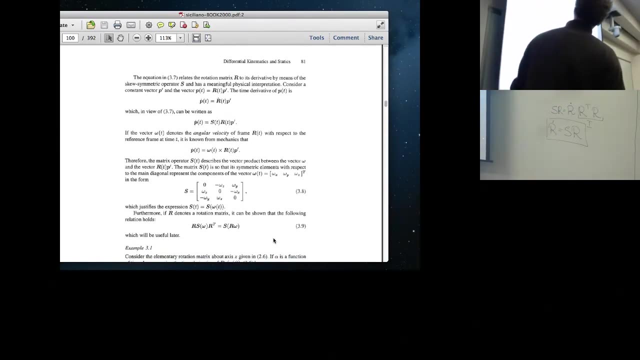 But there's a cheat in there, Because s is something where we also put an r dot inside. So we've got to get rid of that cheat. So Now, what do we do next? Da, da, da, da da. He wants to basically show that s has a meaning which we can interpret in a different way. 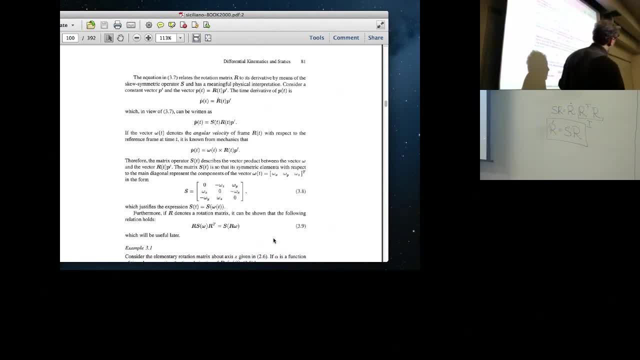 And what we're going to do is we take a simple point which has no offset. We have a point, We just have a coordinate system Which is our world coordinate system, And we have a local coordinate system which is rotated, But otherwise the origin coincides. 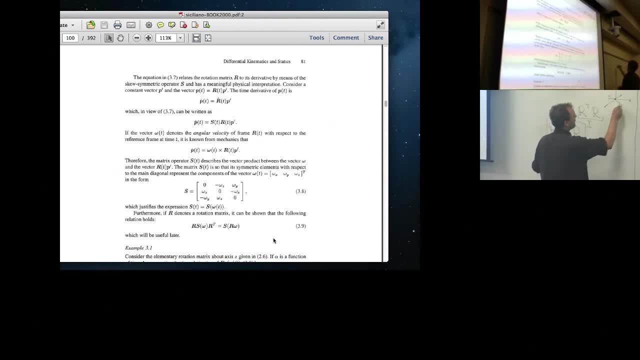 So This here would now be x prime, y prime, z prime. This would be x, y, z. OK. So this is essentially what- And we do say OK. From that consideration we can say that a point p in this thing is going to be r times p prime. 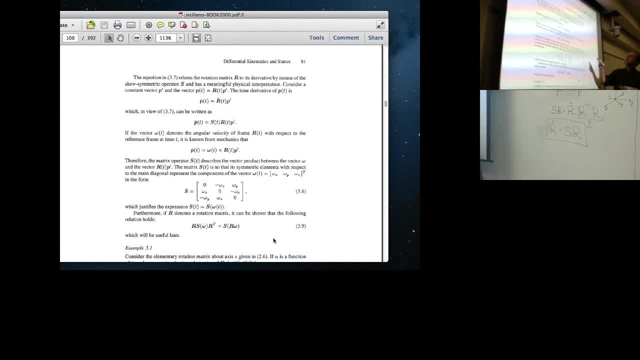 OK, Is that correct? So Good. And then he does this as the time derivative. So what's the p? Consider this: And the frame point is a constant vector, So the vector doesn't change. So there is some way here. 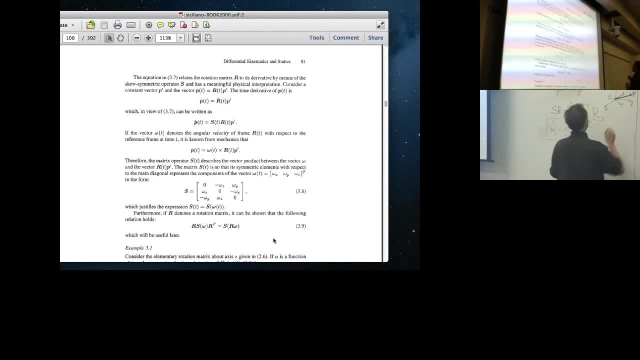 There is some vector, p prime- which does not change. It's fixed in this coordinate system, In the prime coordinate system Right Now he takes the time derivative of that And we just get that. Because p prime is constant, We don't have to take the time derivative. 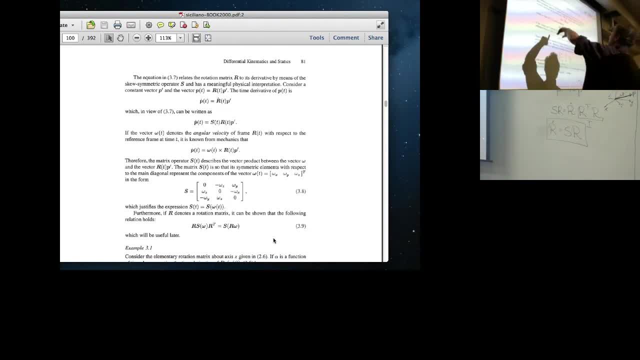 Make sense Right. So- And in the view of 3-7, it can be with p prime. Now we have r dot, Which you can replace with. Let me give you this for a moment here. You can replace this here with s times r. 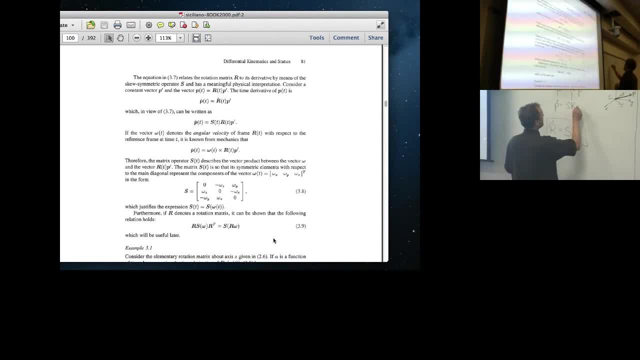 So we have p dot, Well s times, r Times, p prime. OK, Makes all the sense. And now comes. the story is that we can also basically look at p dot from a general point, which we did the last time. So what about that? 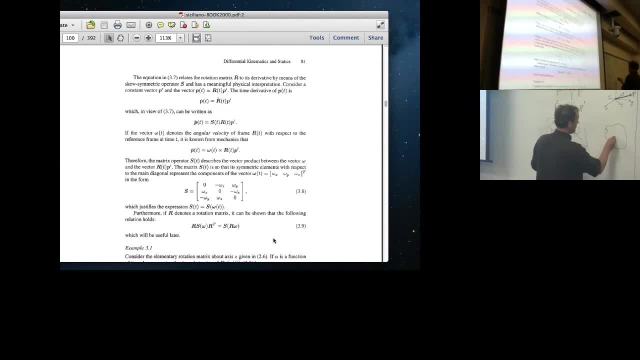 We have a body, We are somehow here on this body And we have the angular velocity of this body, So it's just omega. Let's see what else do we need? And we have a vector, So we have our local coordinate system. 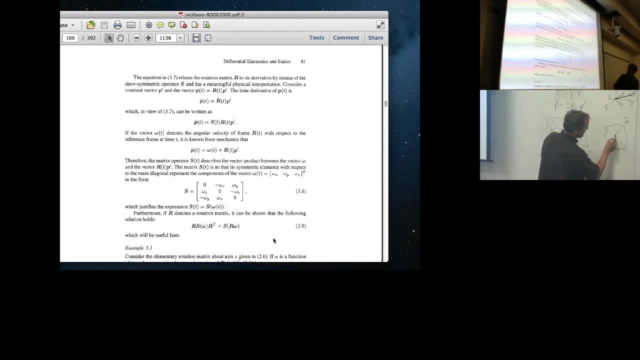 It didn't fit up there anymore. We have a local coordinate system- Let me try to reproduce this: Y prime, X prime, D prime, And we have our vector p, Which is somehow this guy T prime constant here, And we want to know how quickly p is going to be changing if we are rotating this coordinate system with omega. 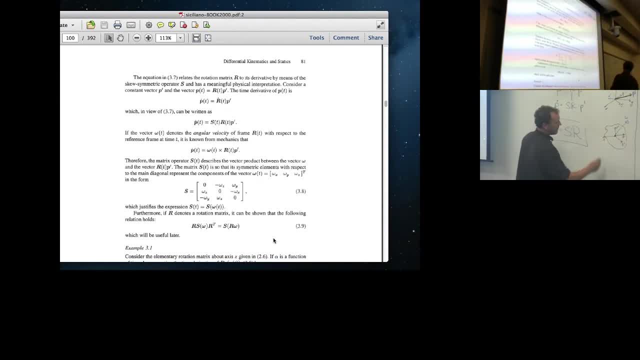 Well, there's a very simple rule. OK, We know how to express p prime in world coordinates. So p prime In world coordinates Just have to be pre-multiplied by the rotation matrix. OK, So now we have to fix the p in world coordinates. 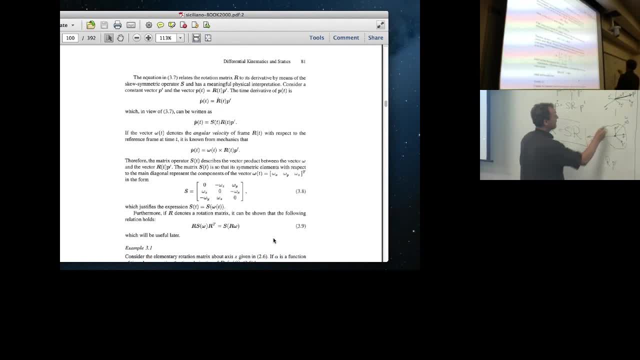 Which would be my big coordinate system here: X, D prime, Y. OK, And now we have basically a vector which rotates at a certain speed with omega, And we actually know that the cross product, The longer cross r times, p prime gives us the velocity of that rotation. 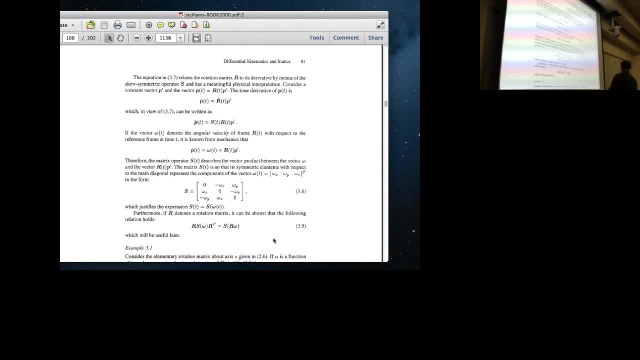 So that would actually be p dot. OK, And now let's say: you see this analogy. So first we said p dot can be expressed like this, And now we said p dot can be expressed like that. And by analogy there is only well, what's different? 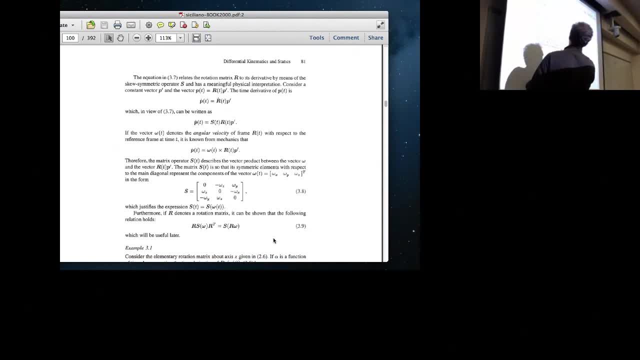 OK, P prime is the same, P dot is the same. Actually r is the same. So we only have s of t and omega of t cross product. You know, we can describe omega of this cross product. We can write it as s of omega. 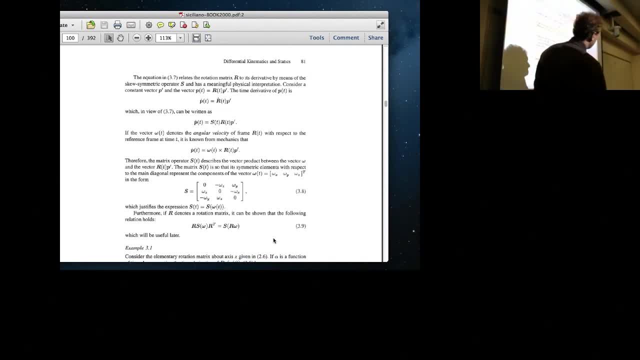 As a matrix. And that now basically brings us into this nice thing that this s here which we've derived, is equivalent to the cross product. That's actually what is the interesting inside of that silly derivation. So we started with a time derivative of a rotation matrix. 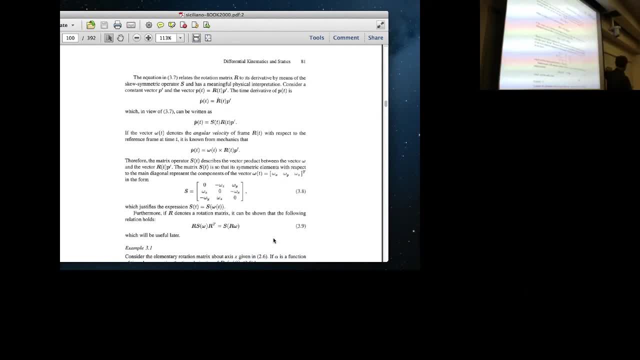 And through some silly substitutions, which usually look weird, we get to the point that we can, by analogy, make the statement that this matrix s, which was, I think, r dot times r transpose originally, is equivalent to some cross product of the angular rotation matrix. 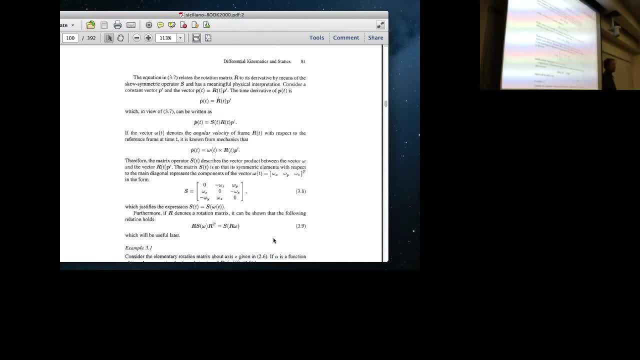 Of the angular rotation, omega Good. This basically now allows us to go create r dots. Whenever we create an r dot, we have a way of replacing it with a cross product Right And before there was a statement OK, s is Q symmetric. 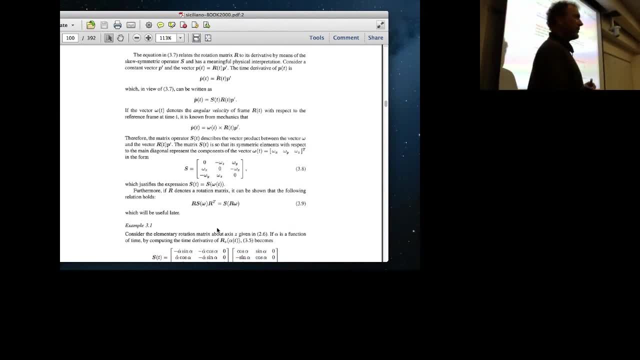 That kind of hinted towards that this could be coinciding with a cross product. Remember, we wrote at some point: OK, S transpose plus s equals 0, which only holds for Q symmetric matrices. And just know that the replacement of omega with a matrix is a Q symmetric matrix. 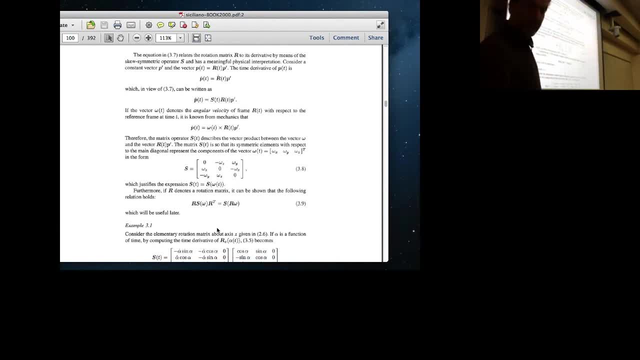 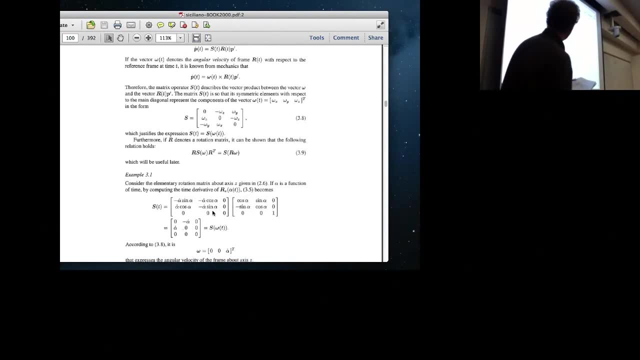 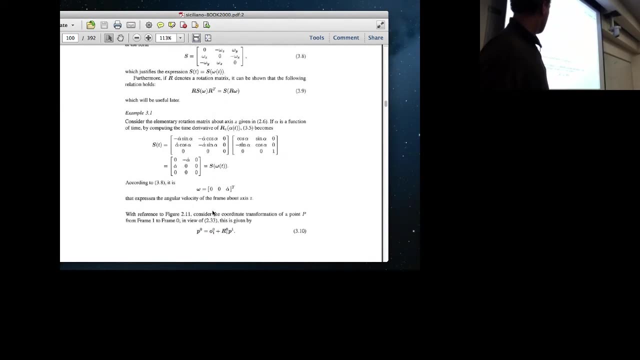 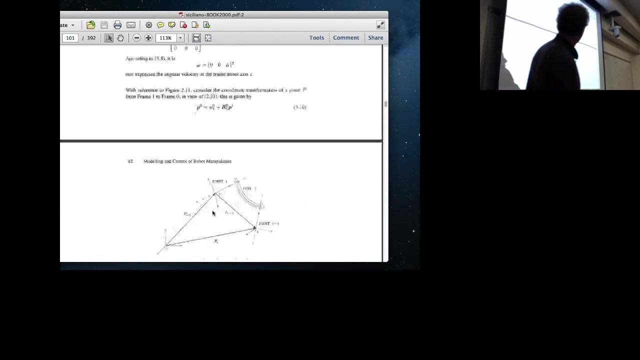 So we have this all sorted out And we're happy forever after, And we basically- well, we can do all kinds of substitutions. Let me not go through those things, otherwise we'll run out of time totally And move on. So we want now- and I'm not going to go through all the glory, since this is coming too much- 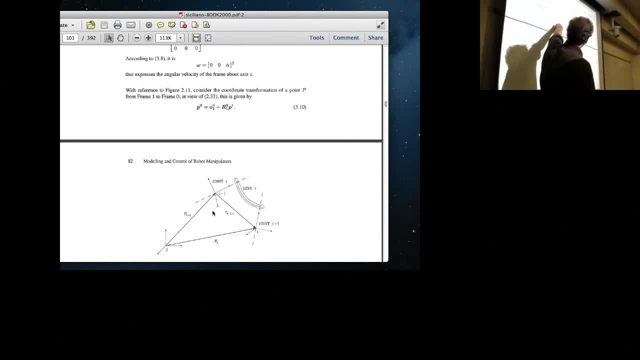 We want to now go back to this idea that we have a point in a local coordinate system. We have the rotation matrix and the offset. You could also write it as a homogeneous transformation matrix, in case you remember. We want to take the time derivative of this thing and see what happens. 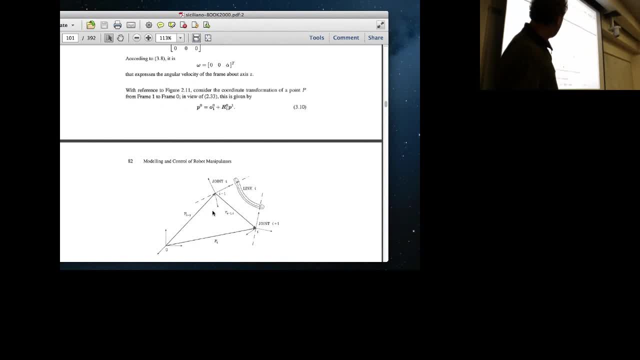 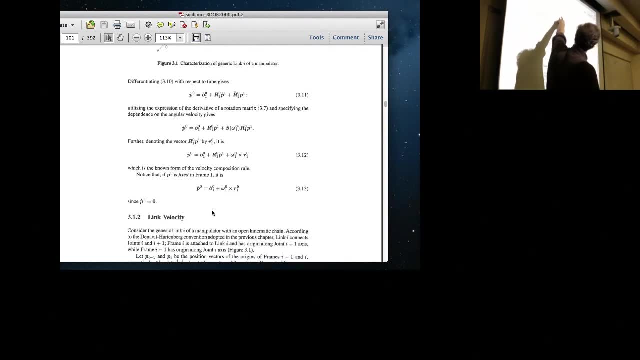 OK, And I think here we can just look at what the book is doing. So time derivative: again, We use the chain rule. It's p dot o dot. This is easier than r times p dot and r dot times p OK. 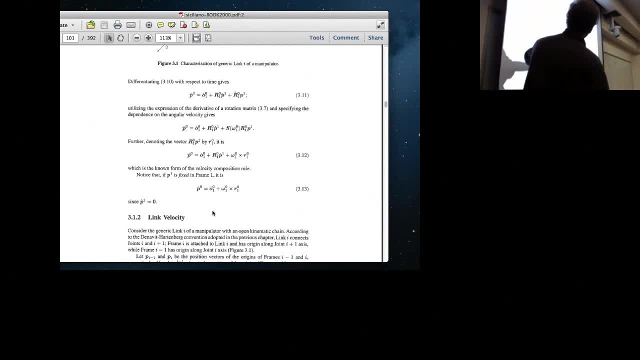 Very straightforward. I don't have to write this again. But now comes the little trick that you can basically replace r dot here with s omega 1, 0 of r. That's the transformation from this. It's a world coordinate system. That's what we're applying right now. 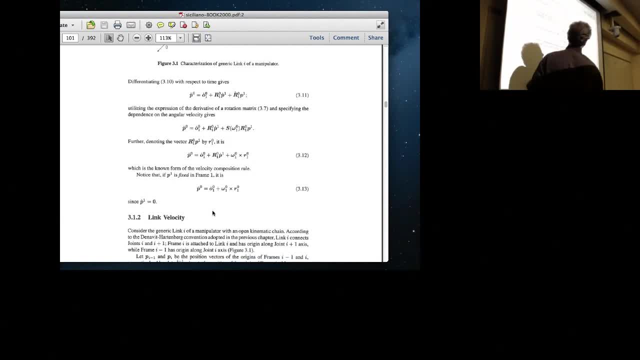 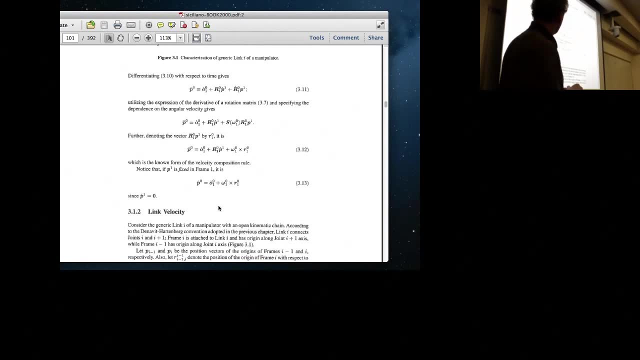 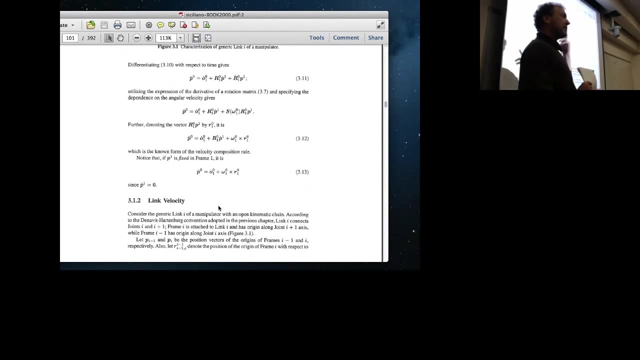 OK, And then we can write this here as a cross product And we're kind of happy. And then it's basically he just says: OK, if p expressed in the local coordinates is actually constant in the local coordinates, then its time derivative is going to be 0 and this term drops out. 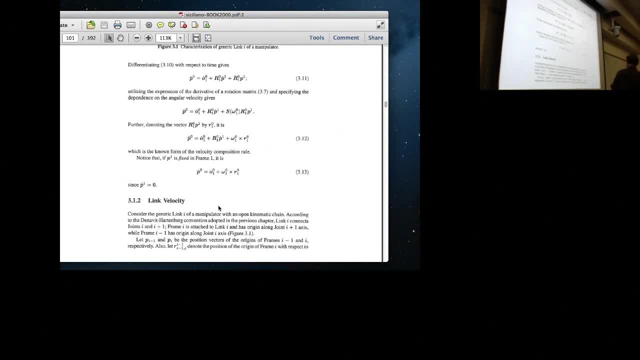 So what you will see in Newton Euler is that- let me get rid of all this glory here. In Newton Euler we have multiple links, which I just now tried to draw Very simple, And we try to express things like the center of mass and other quantities with local distances like r. 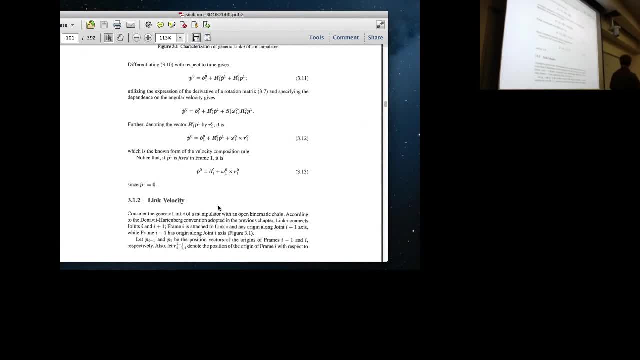 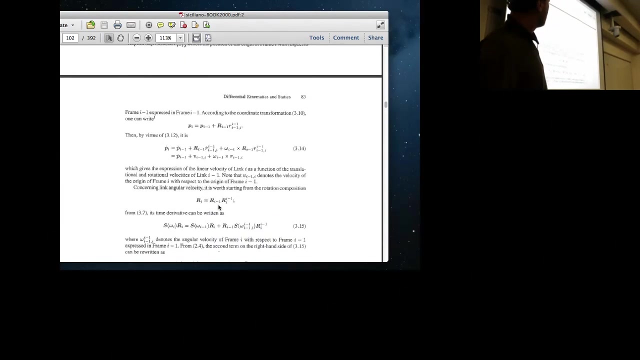 OK, So we have these things which are fixed in a local coordinate system all the time, which is why we very frequently can drop these terms out. Actually, we will never see them again. OK, So this was the generic rule And now he basically applies that to link velocities by creating a recursion. 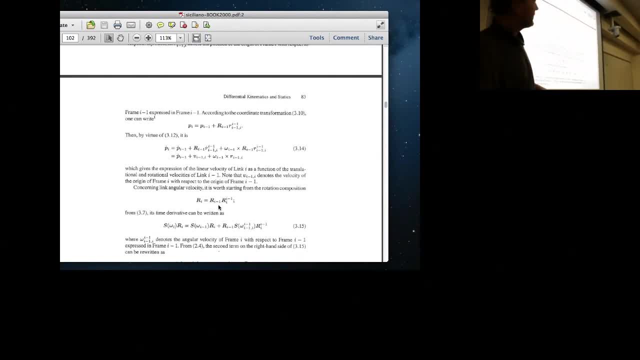 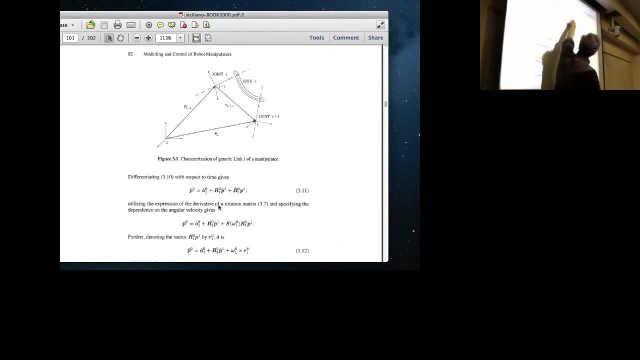 Same story as before. So let me see, here We have a. yeah, We must have a plot which was higher up. So this is basically now the picture which we're working with. We have one linked i here, We have its axis, its joint, yes, joint i. 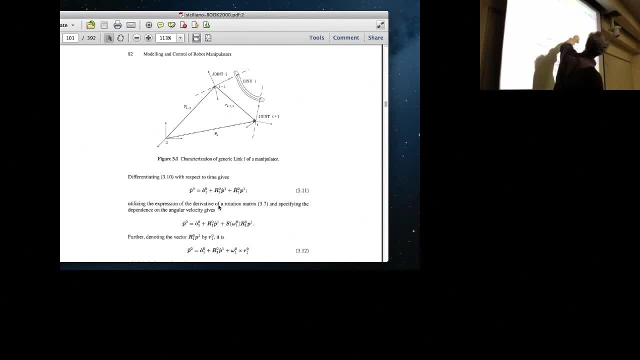 And here's basically point i minus 1.. Here's point i. Here's the vector which goes there, Here's the vector pi which goes there, And then there's locally kind of the distance between those two guys. Oops, The vector r. let me just write this: r i minus 1, i. 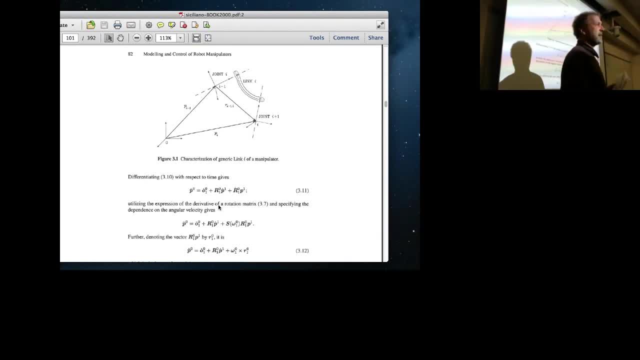 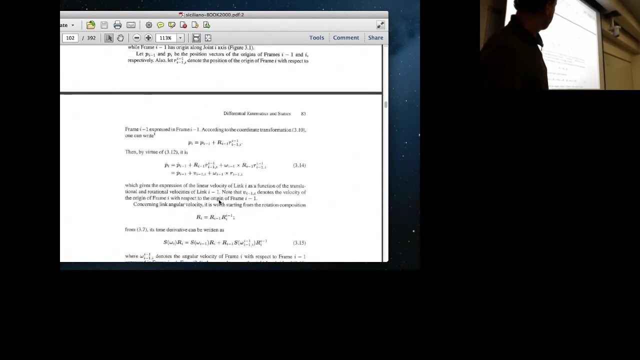 Now, as you notice, the subscripts and things become a little annoying. Cool. So if you have this picture in mind, then we basically just try to express link velocities by a recursion from one link to the next, And that is essentially what this stuff is supposed to accomplish. 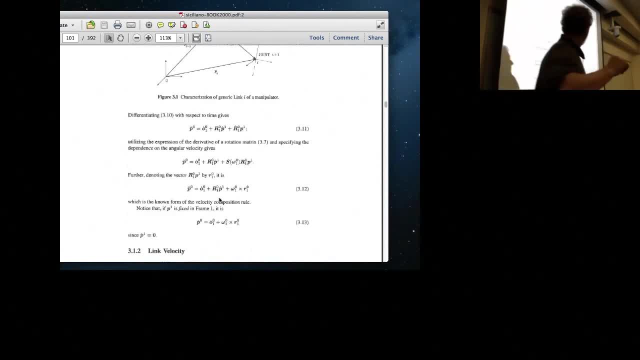 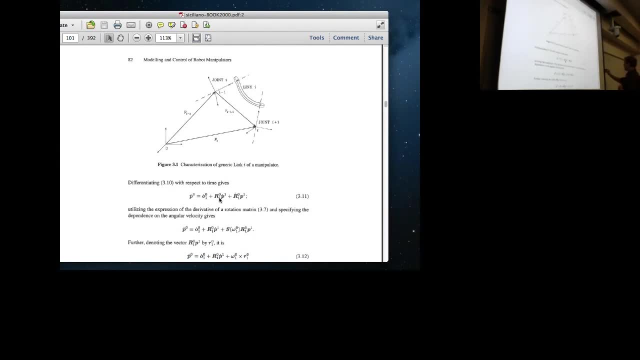 Let me, maybe we need that picture. Let me just reproduce this picture real quickly so we can refer to that for a second. Okay, So we have coordinate system here And we call this the world coordinate system, And we have, yeah, 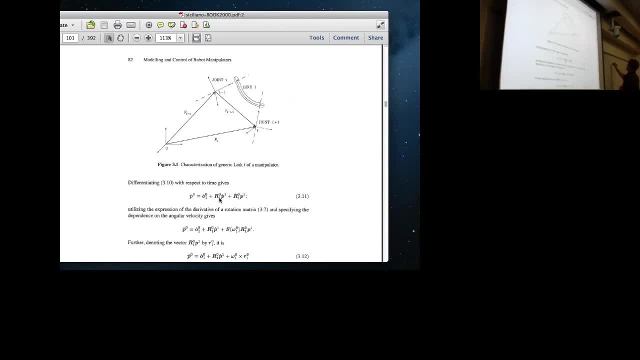 A point i minus 1.. We go here to a point. This is kind of i. This here is pi minus 1.. This here is pi. We kind of fantasize that this here is kind of our link somehow, or related to our link which we care about. 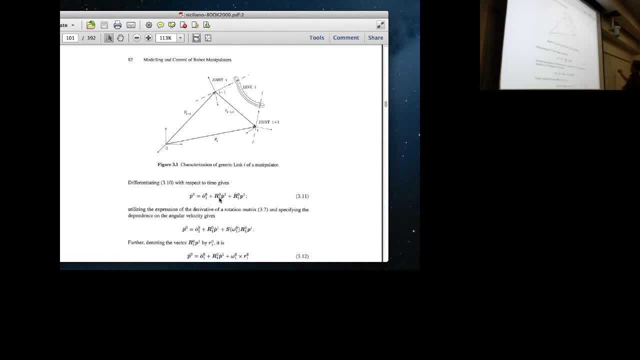 So this is link i And you just hand it out there because it's easier to draw, And we have this offset vector here which is going to be r i minus 1 r to i. Okay, And as long as there is no superscript, it's all expressed in world coordinates. 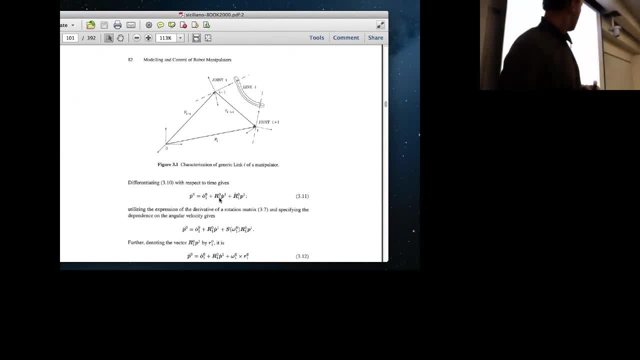 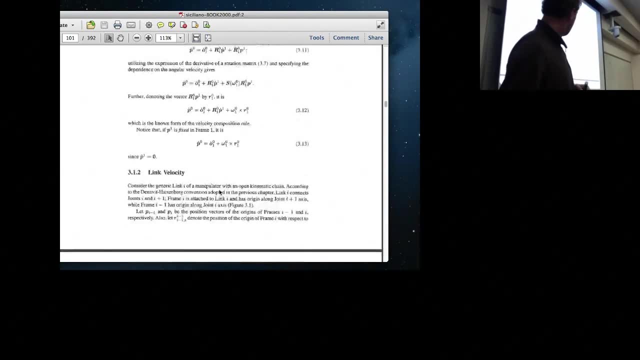 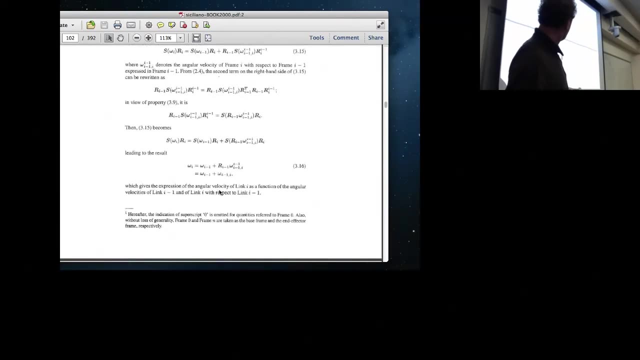 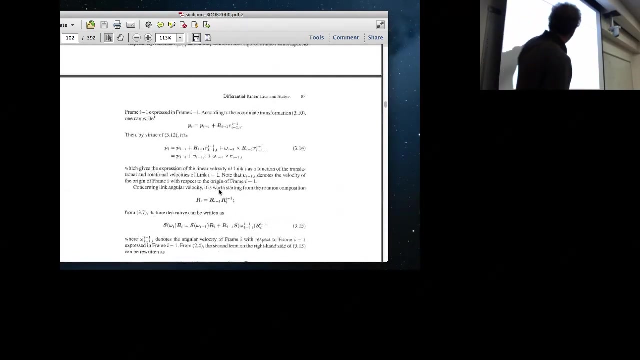 Okay, I think I have all the notation we care. So then, basically, in this we no, where am I? I'm completely hopping around like crazy, Sorry, Good. So now we say pi can be expressed as pi minus 1 times the rotation from the i minus 1 to i. 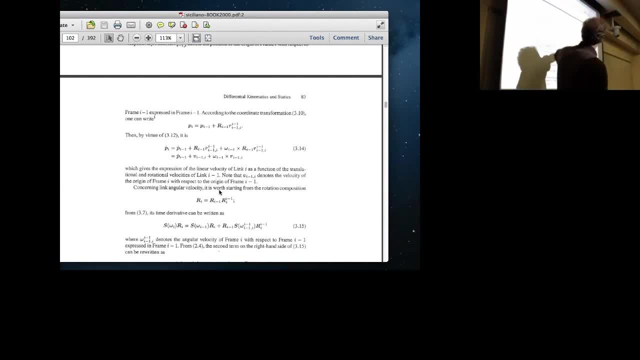 Okay, So i minus 1's coordinate system times this guy. Okay, I don't want to write these things a lot, I'll write it one time, So much fun. So pi equals pi minus 1 plus r. So the rotation matrix which takes me from the i minus 1 coordinate system to the world coordinate system. 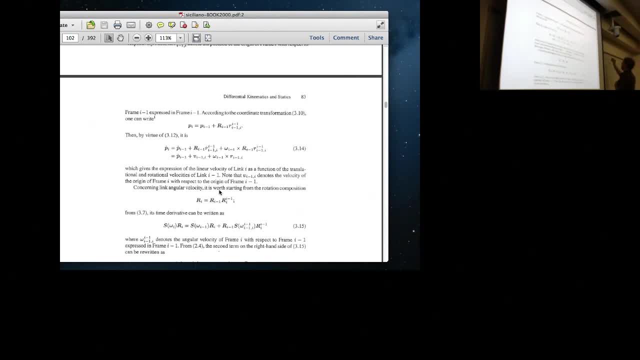 And I can put the 0 up there. And then now comes the notation becomes real fun: i minus 1, i. So that's the distance between these two points expressed in the i minus 1 coordinate system. Okay, Fun. This is why you have to get the rotation matrix. 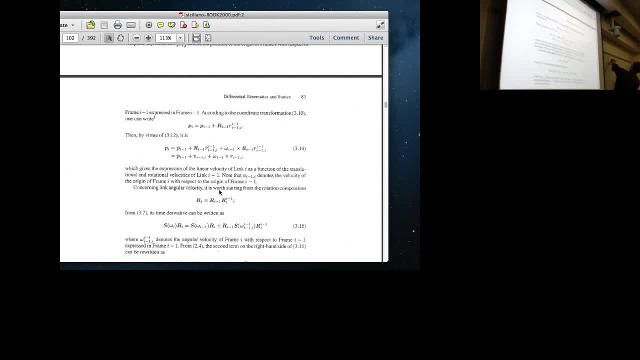 So basically he expresses this distance in this local coordinate system, So that becomes now a constant in this local coordinate system And he rotates it in the world coordinate system And adds that offset. So it means this vector plus this vector gives this vector. 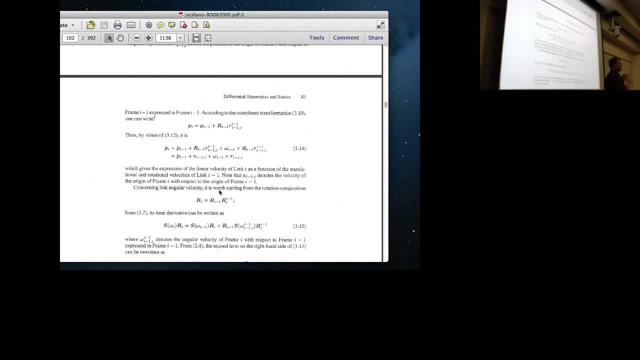 In the end it's totally straightforward. It's just notation wise becomes a little bit unhappy. Good, And if you believe in that, all we're going to do now is differentiate And we get exactly the same story as before. So we get all these little terms. 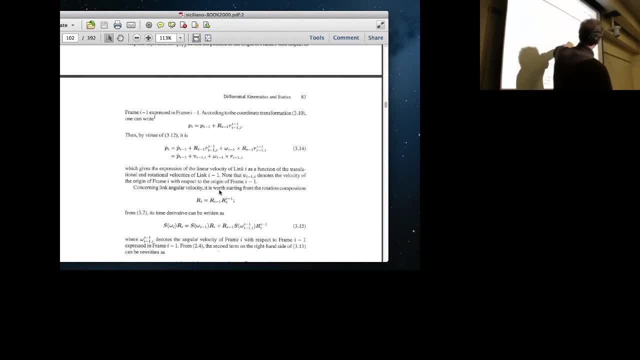 We get a p dot, We get an r and a little r dot And then we get the r. you put in the substitution with a cross product Where we got the matrix derivative, the rotation matrix derivative, And in the end we end up here with this equation. 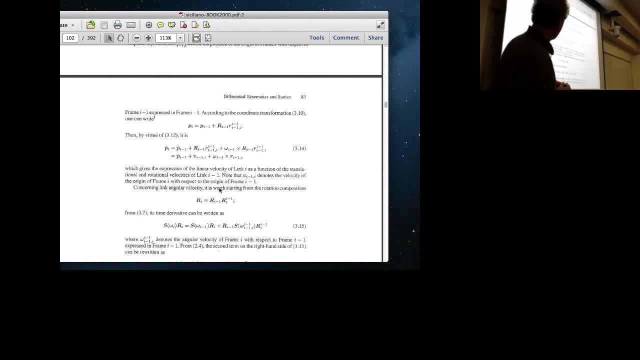 So this is just the general expression And that basically still assumes that r dot might be changing. He keeps this in there for the one reason that if this happens to be a prismatic joint, we would need it. If it's a revolute joint, we will not need it. 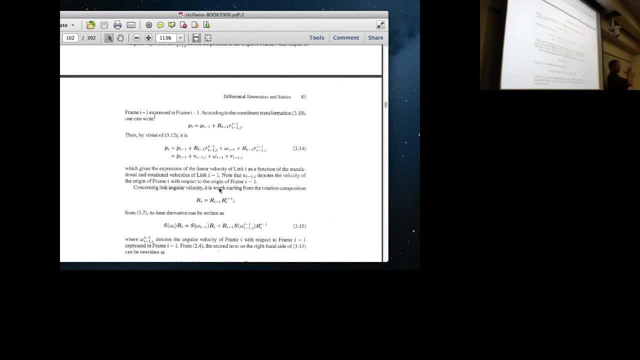 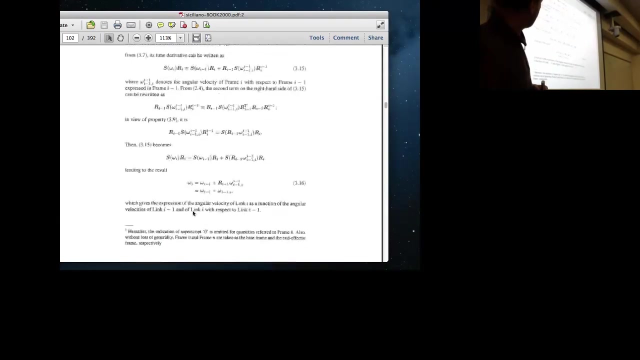 And he's going to drop it out later when he basically discusses the difference between prismatic degrees of freedom and revolute degrees of freedom, But he just leaves it in for a tiny moment. Whew, Okay, Let me just move on. I don't want to go through all of it. 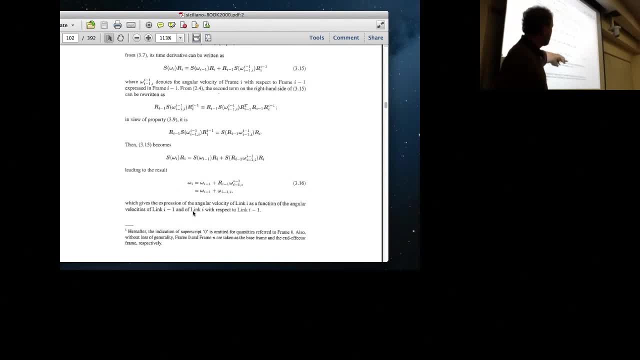 He does the same story for rotations, Which is actually Much easier. Rotations just add up. So omega i, The angular velocities. I should say Sorry, Angular velocities are simply the previous angular velocity plus the next angular velocity, That's it. 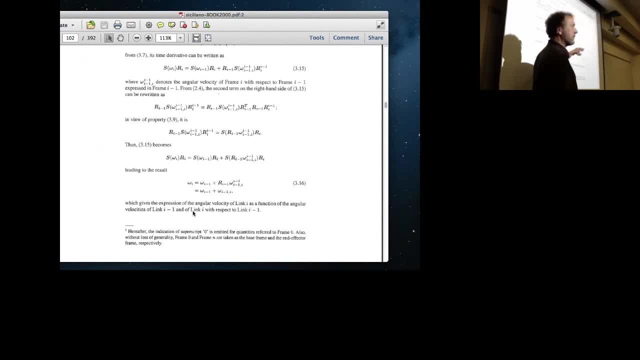 Now expressed in world coordinates, Or here he expresses one in local coordinates. So this angular velocity in local coordinates would normally be the velocity of this particular degree of freedom, revoluting, Okay, And if there's nothing rotating, it wouldn't exist, potentially. 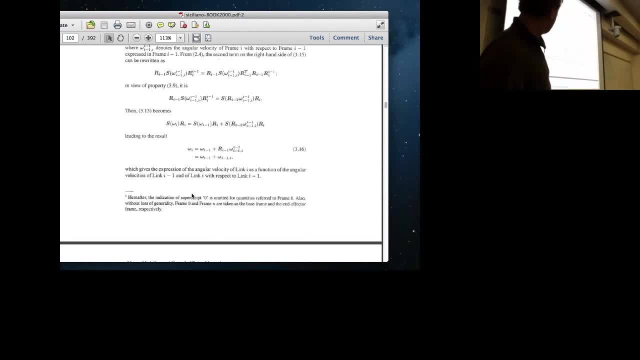 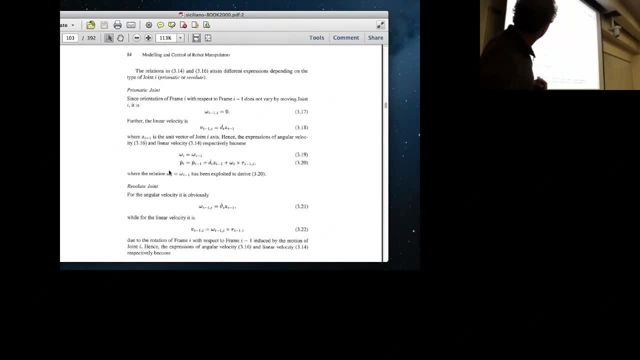 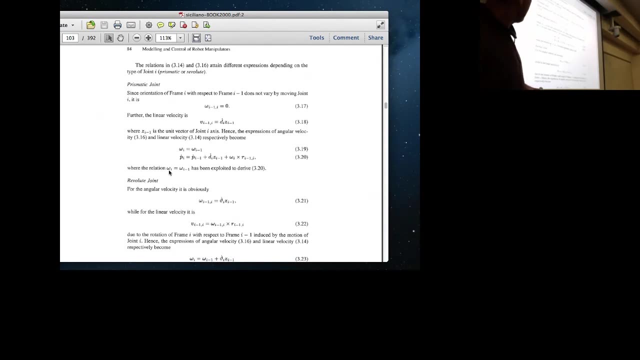 Good, So there should be a summary of that. It's becoming too much fun. Some of my fingers don't work today. Okay, Here we get. What do I want? That is a kind of what really matters in the end, All the things which you would like to. 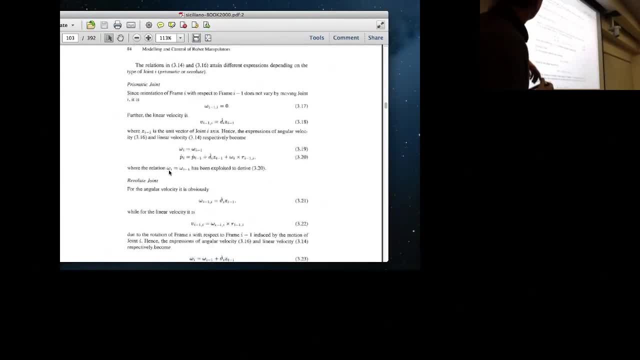 Come on, A little bit more fine control would be good. We basically now differentiate between prismatic joints and revolute joints and get rules how to express the Angular velocity and Translatory velocity Of a particular link. So very simple: prismatic joint that doesn't rotate to zero. 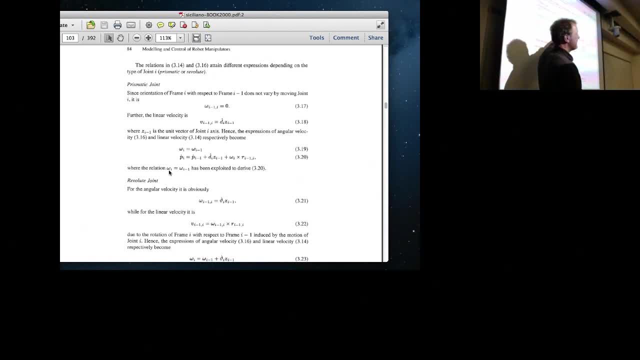 In my transitory velocity. Basically, He uses the d dot, The change of d Times, the direction of the axis in which it goes, Plugged it in to get that formula And for If you have a revolute joint, What you get is something which looks like this: 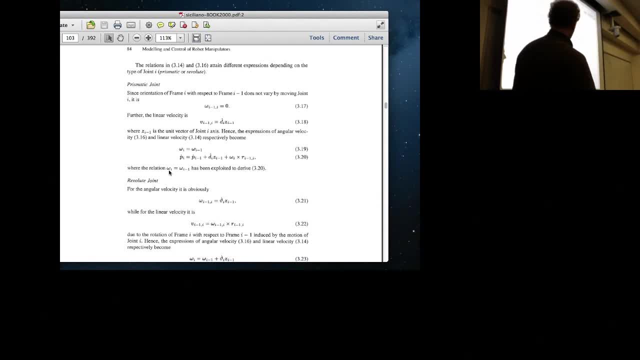 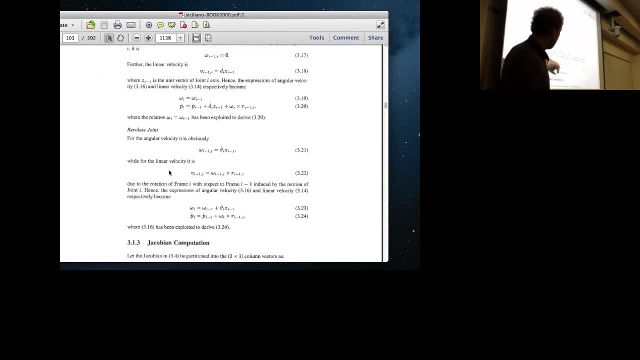 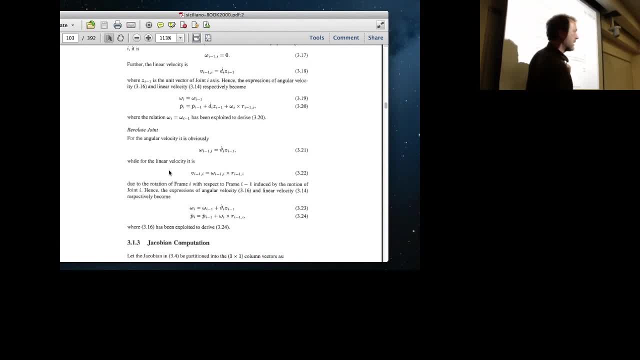 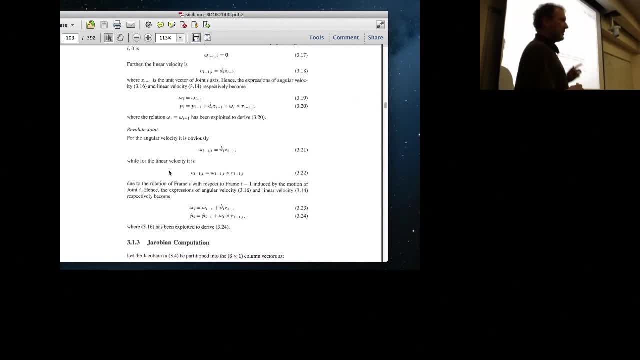 This And this, This, The Same conditions Of olo3.. So You Got screamed at you here. That very important. if you would sit down and do this carefully and think through every of these darn indices, whether they're sub or super or whatsoever, and 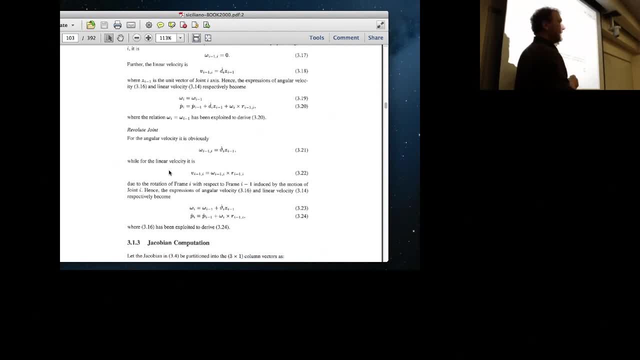 have that little plot in mind while you're doing it. it's not very hard to follow when I'm talking about it. potentially it might be sometimes confusing- just talking about these indices is confusing, so- but it's not very complicated. it's a very simple geometric argument: how to make forward. 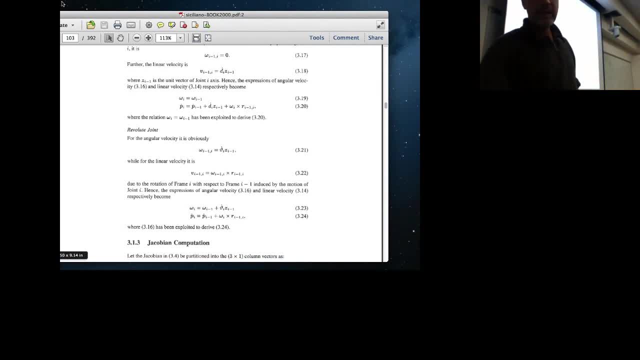 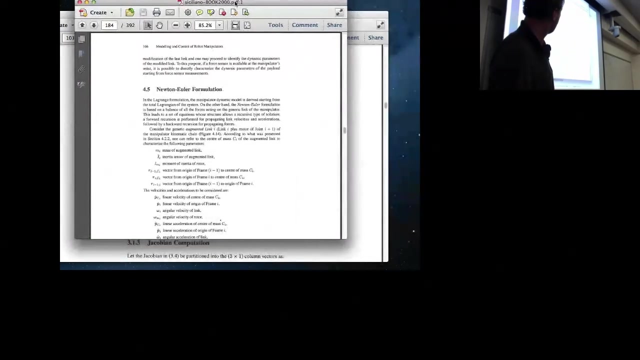 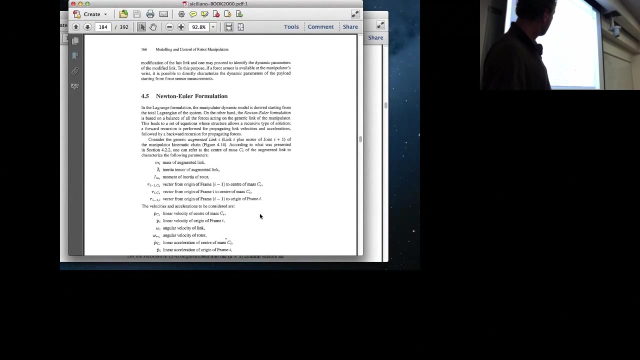 progress good. and now comes the next big picture which I want, and if make it my mouse pointer, let's do Newton Euler, because it's so much fun and my entire existence will be about explaining one plot. okay, this is all the notation he's using. you could read to that, but you can actually try to. 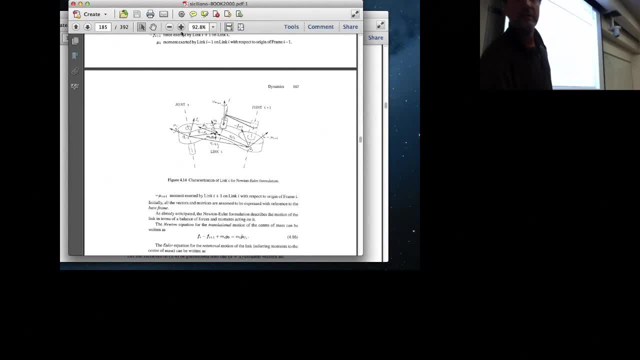 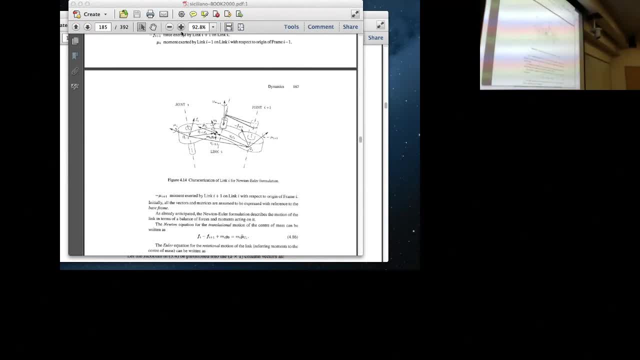 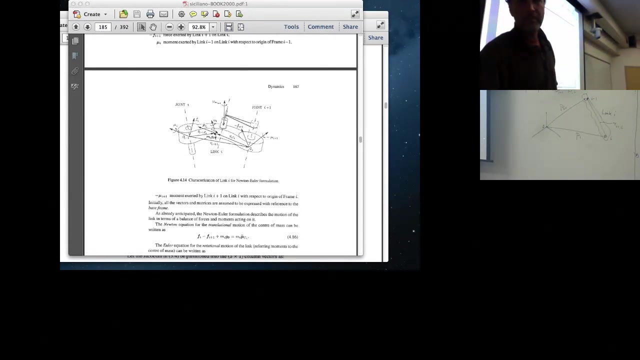 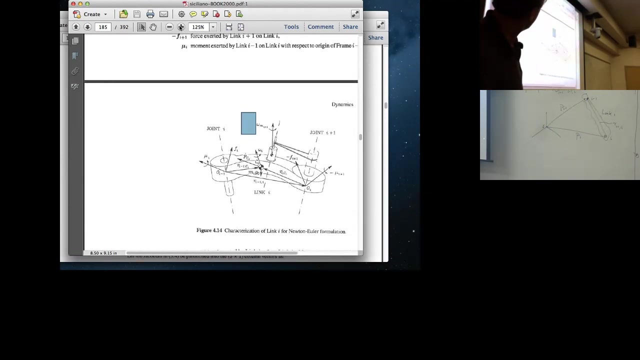 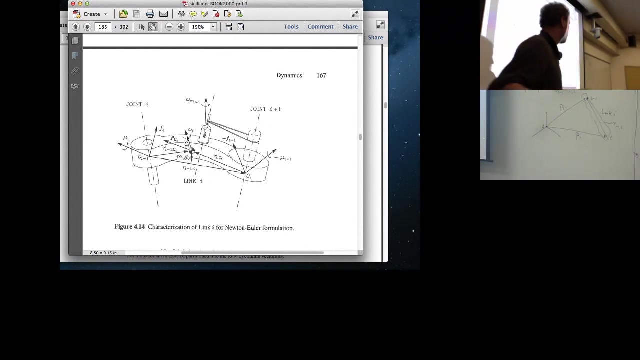 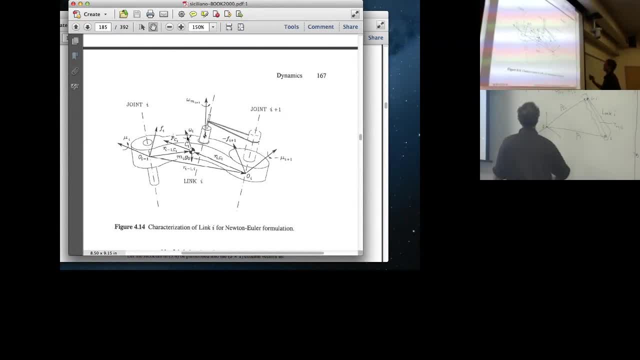 and notice, when I draw it one by one it becomes actually very simple. so we take our favorite little think picture here. then we're this hole here. have to make this somehow 3d looking better. so we have the rotation axis of joint I one, and here 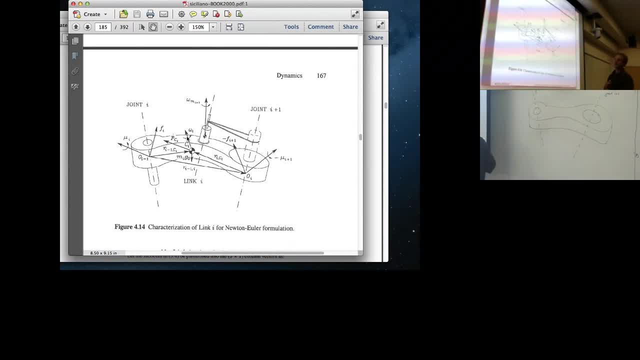 join. I cool, then what else? you don't need so many things again. I skip everything which comes from the motor which will make this more clearly, that picture, easier to understand. so we have one coordinate system here which is Q I minus 1, and then he puts no, oh sorry, so the Q O. 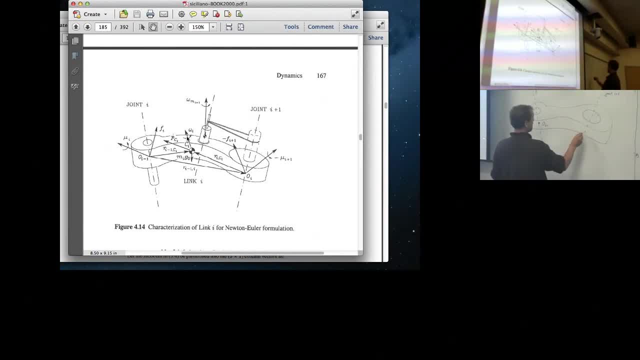 orange, and there's another one here which is all I, so I don't put in the coordinate axis instead of finding, and we have somewhere a set of math which we assume we know in local coordinates. now, the distance of the center of mass from this point of view, from this coordinate system here, then becomes our I minus 1. 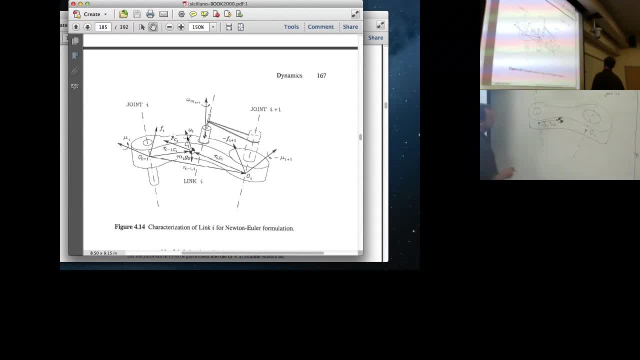 to CI, the center of mass, and you can also write it equivalently, like up here: it would be R, I to CI, and we have at the center of mass our good old friend gravity acting, which creates SI times, G, and G is zero, because it's either, I call it G. 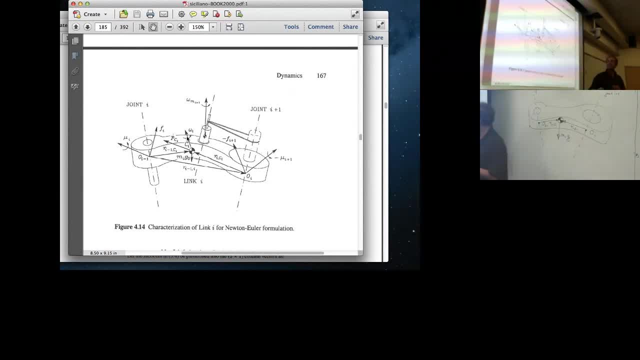 or I call it G, but most likely he means that. okay, and we have the entire link on the thing before. all right, terrible is just fine. from here to there is R I minus 1 I, as in the previous picture which we just had. good, so this is. 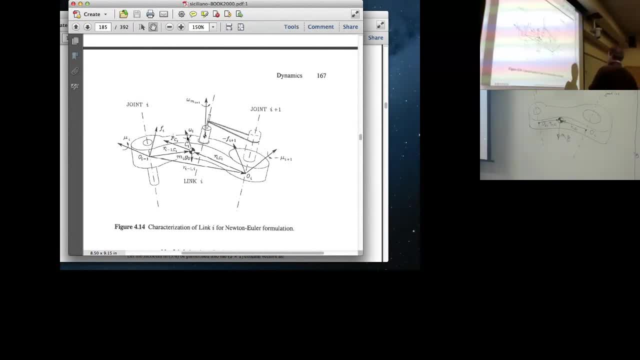 kind of sitting on the tree of this now and to balance what happens in all forces of momentum, you know, is every general way. okay, I'm simply say that here has to be a momentum which we call my I plus 1. back to the, The other momentum on the other side. I can't even talk about this. this is called new eye. 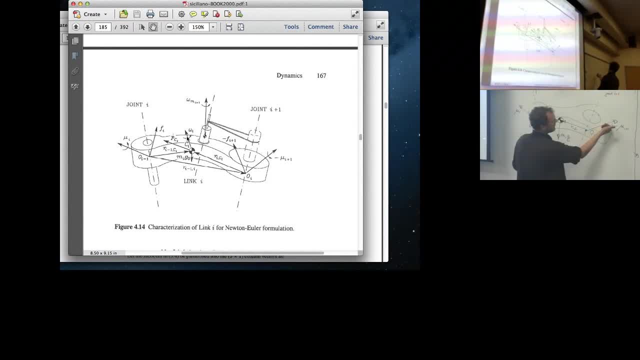 The rule is always: right hand roll. you stick your finger into the arrow and that's what's called a positive momentum. So where do they come from? A reason is to cut it out of a roll. Okay, here's a big roll, let's take me for it. big roll. 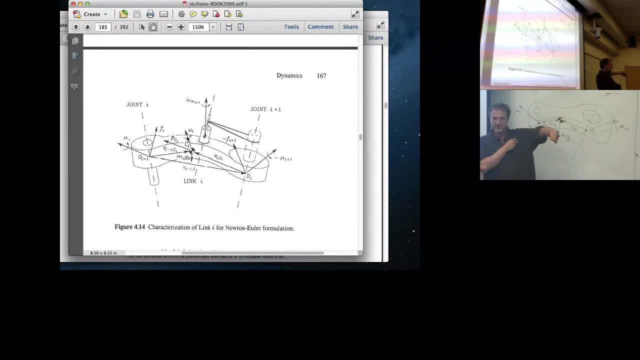 I'm going to consider my arm and cut it out, discarding this, But not changing about this. you cut my. you have to put in forces and force that my upper arm stays there Same on the other side. You just need to cut it out without changing the position or anything of this link. 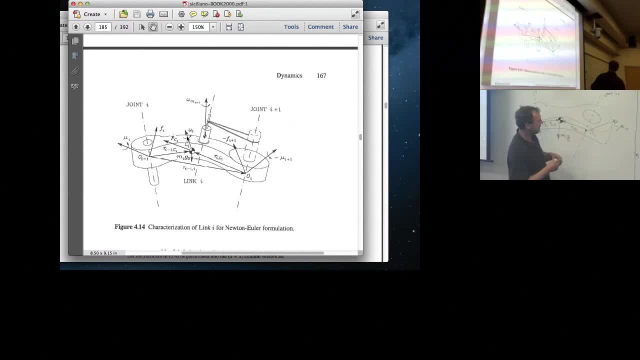 So that's basically it Momentum Afterwards. and the interesting thing is, if I put the other one in the momentum and the forces have to balance each other- That's what Newton told us at some point- We always have to have negative force. 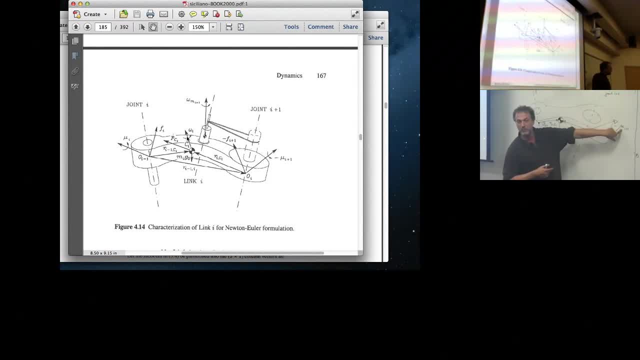 The other link on the other side would be plus mu 1 as the momentum And if you put them together they would just balance and everything would be happening. This is why we have to do new eye, New eye. The negative force minus 1 again. 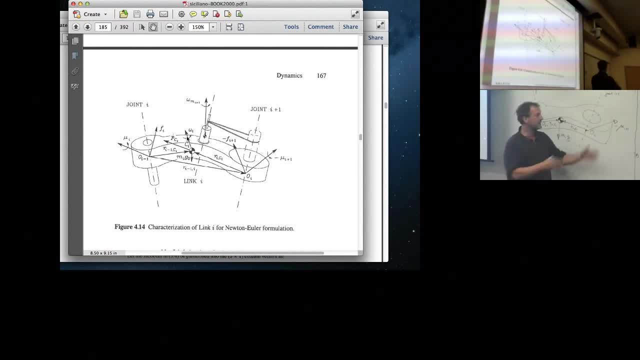 On the other side. they have to have the negative sign, Otherwise they wouldn't put everything together. If you can't have all of them, That's it, I don't know. All right, we do the same thing with forces. It's the same argument. 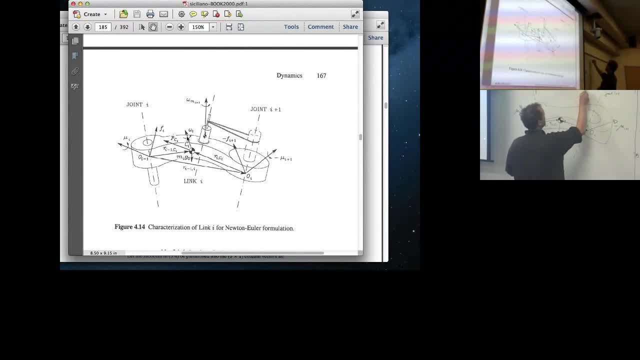 We have a force minus just 1 that we can inherit from the link on the right, And our force here locally is going to be minus 1.. And our force here locally is going to be minus 1.. And our force here locally is going to be minus 1.. 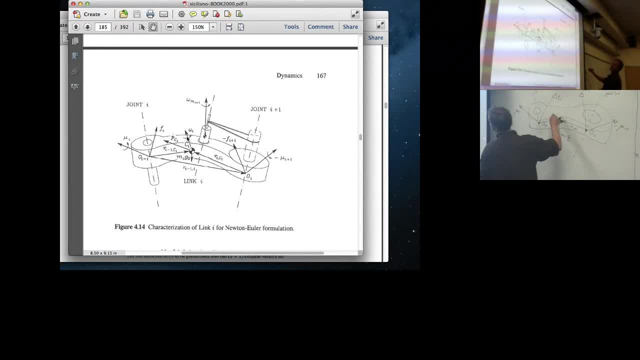 And then we, just This little thing, is doing what It's rotating with omega i. This is this guy And it's translating at the fellow map with p dot ci. How is it that the right-hand side is negative? The force is negative in the moment? 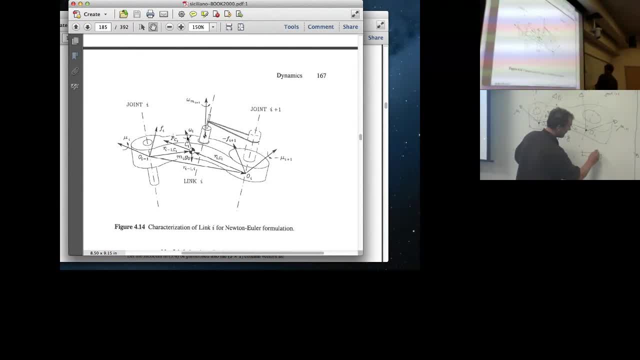 It's very simple. These tulips make a strange springboard swimming pool. This is a swimming pool, Water Blue jumpers jump And normally here jump. Now, if I want to do things up here, then the original force from this will be pushed. 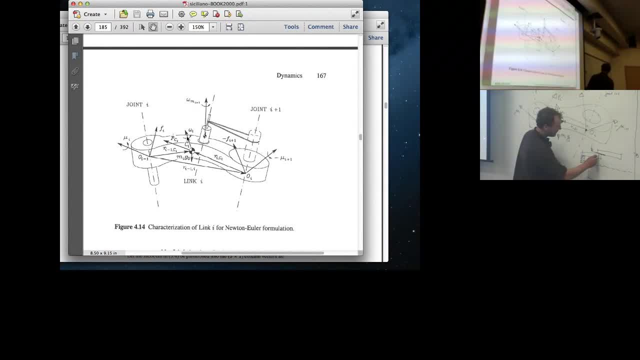 And according to this, there has to be forces up there to counterbalance that. Let me do the force here, And then there's a force here, Let the two counterbalance. We basically just What comes from the next link here And we put a negative sign on it. 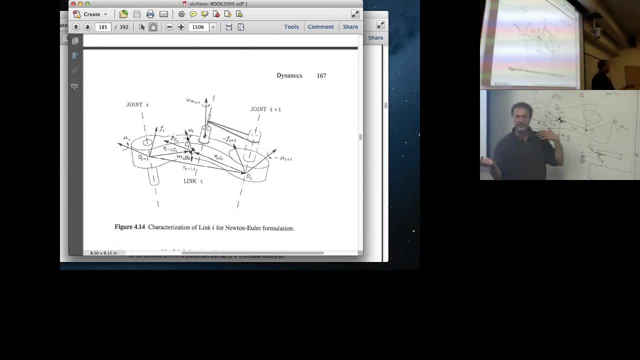 Because Positive on the negative, It could change that. Cool. Now all we got to do is we write force balances and torque balances Since going to Mr Newton, all of those and Mr Euler. they have to basically sum. 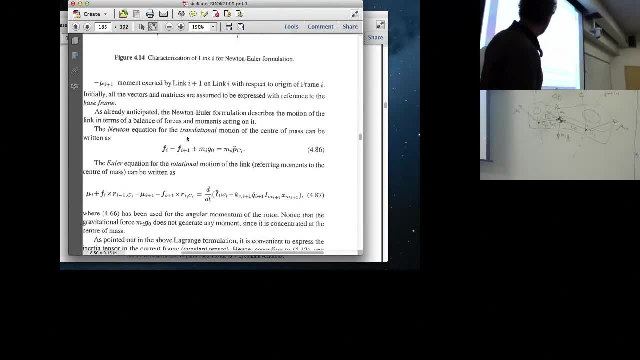 So here's what we do with force balances. It's now very straightforward: You take all four, So force, You're going to have only three forces. Da-da-da-da-da, I is Minus One Plus. 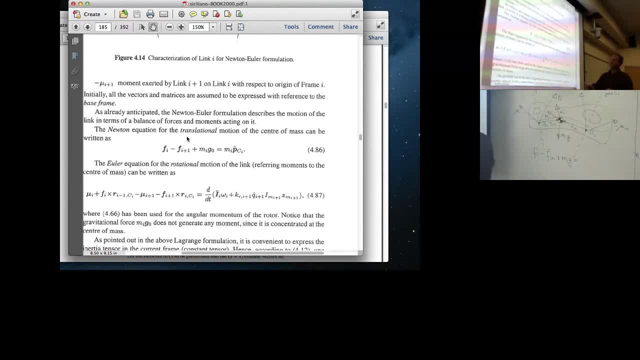 Mi times g, And You can, Mr Newton. this has to be equivalent to The mass acceleration Of It. is that? That's a fine mu And This, And we have to do the same thing for Oh mental. 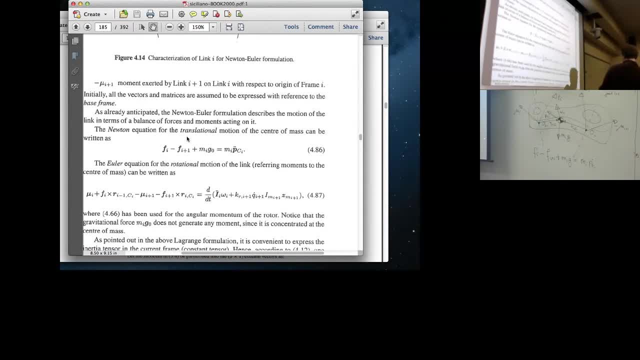 What is it? D There's. well, I want to tell you that part later. Alright, You can see how to recruit. Well, this tells me how to express the force Fi, based on qualities which are local to me. This is the length. 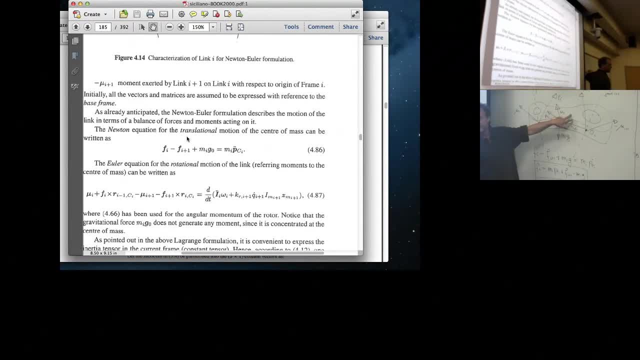 This is the mass, This is the acceleration And the gravity, which is great, Plus the force. If you have a robot, you go to the. There's no connecting link anymore. I thought I can compute the previous Fi and then I can my way down. 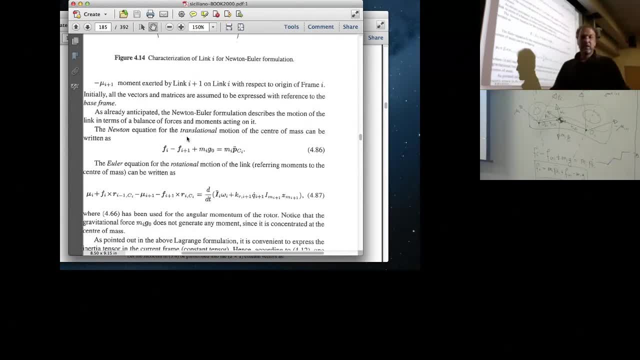 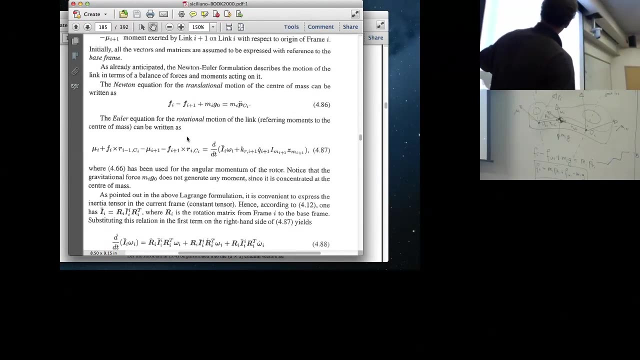 Quick check. is it time Doing okay? Um, doing the same thing for momentum. And he puts always motor stuff inside and we try to avoid that if possible, Because you have motors behind the inertia components. He has the motor components, Everything. 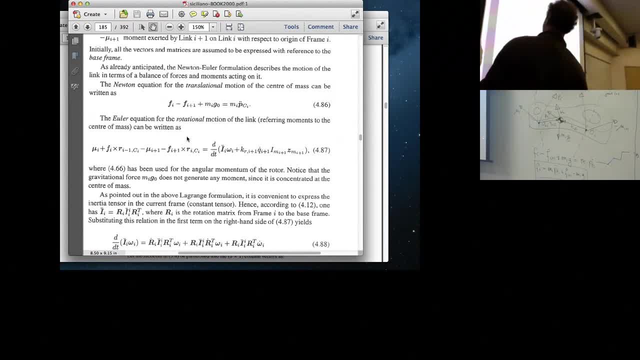 changes a little Him. he just skips. He doesn't need that. So the momentum is much more complicated, but not much. Yes, And you ignore it if you don't care about it Right now. I don't want to care about it because it creates too many terms. 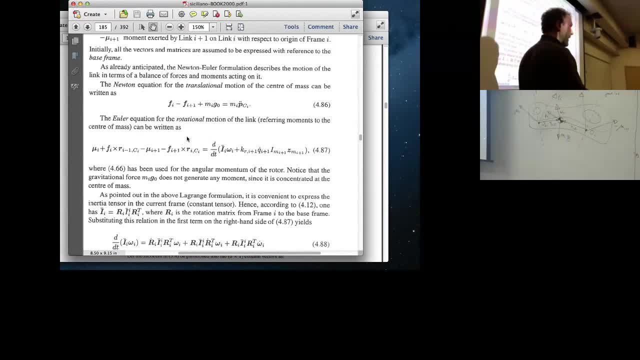 And it just replicates other terms which are just more math and novel insights. If you want to model a robot properly, you would have to put them in. But you can also. often you can't If you make all the math parameters. 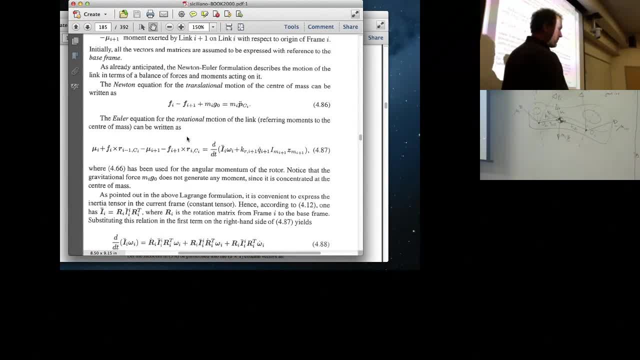 it doesn't matter, It's a big, It's everything together, without explicit modeling, the mass, the motors. So that's what most people do Try to do: the So momentum balance, same idea, So we get mu, i is one. 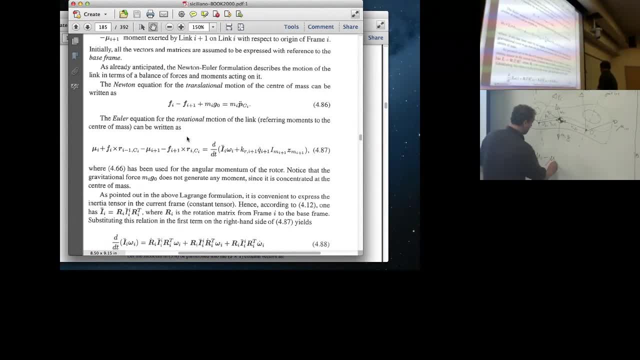 Then minus one, That's one. These are the two momenta, So we have them here, But then we get additional ones from the forces. Remember You do a momentum balance. When you do a momentum balance, you need a reference point. 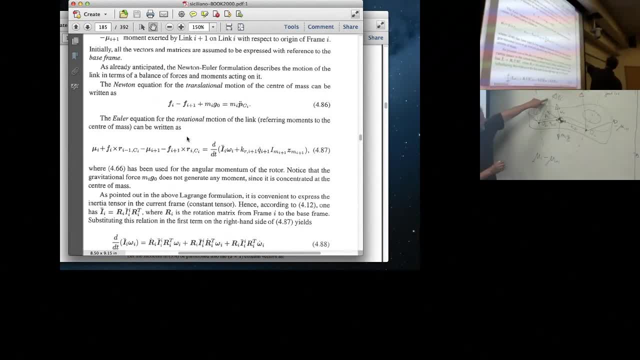 And we use the center of mass as a reference point. It means actually the force F with a distance like this. This is the same idea of the springboard. again, You're standing here on the springboard. It means at this point here, where this thing is attached to the concrete. 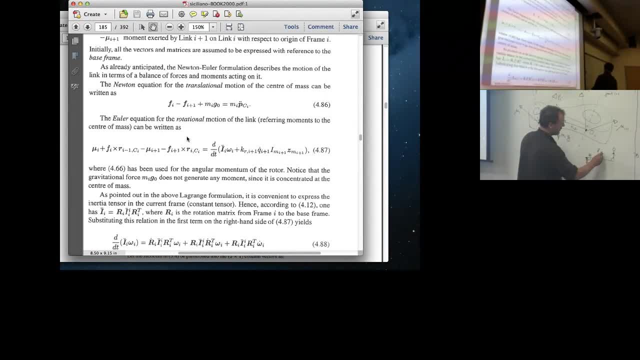 the inner momentum is going to be: F- cross your weight. That's the difference. And you cross it, That's your force. state of the springboard: Okay, And that's what we're going to do right now. So we basically simply say F- i. 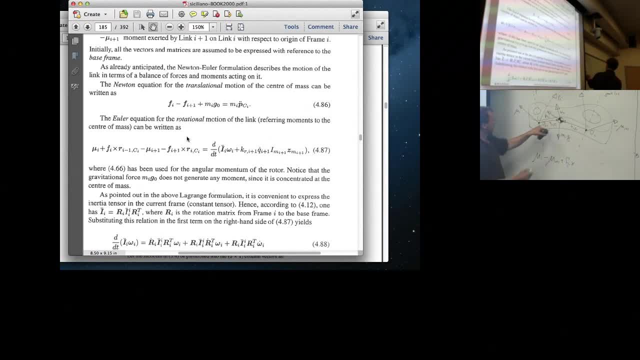 Cross the offset with the distance to the Mass, Which is R i Ones, And I hope I have this term now correctly. That creates a momentum And then we have to do this from here. That is F minus one for a spring. 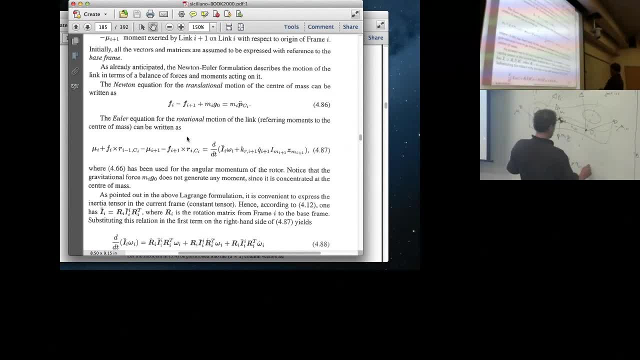 And it should be So. minus That's one Cross R i, i, And this has to. Well, It's a change of, Which is the same equation Derived as T Of the change of momentum with i times omega. 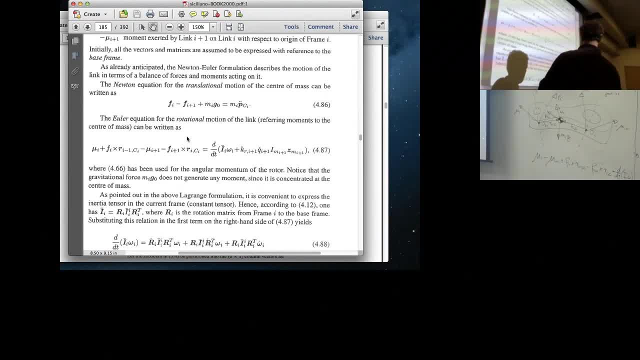 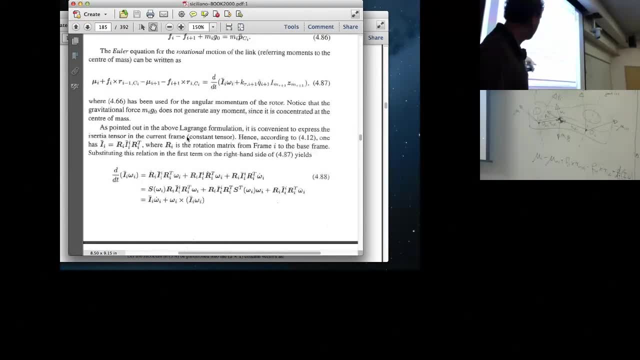 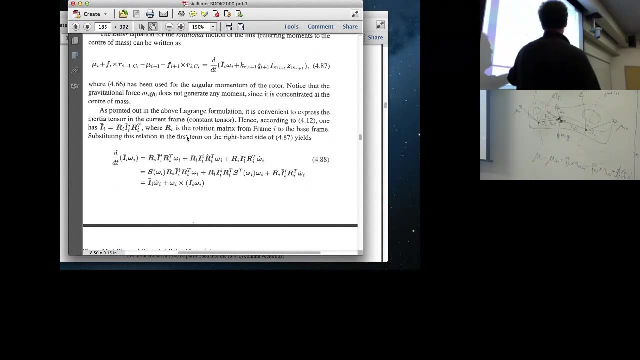 That's the inertia, And we forget all the other terms. And then he basically quickly shows that that basically results, This type of derivative results in this formula. I'm not going to go through this. It's just an exercise of Zero, this matrix. 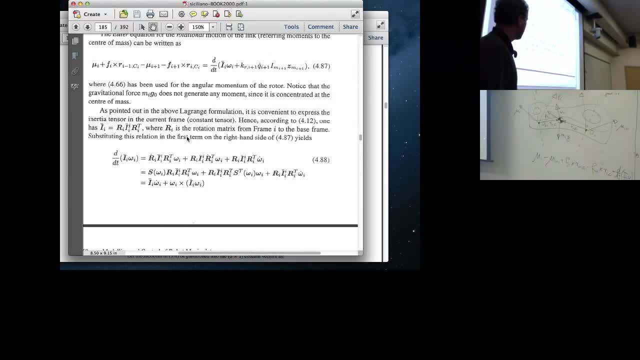 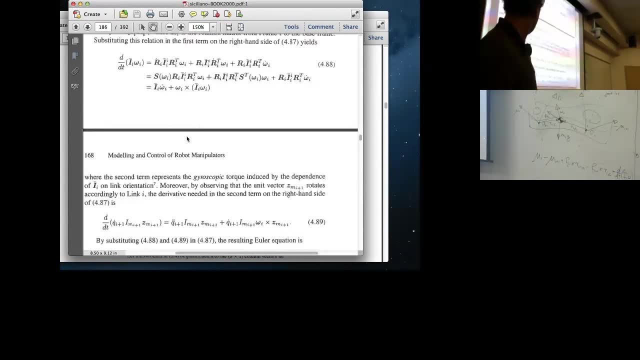 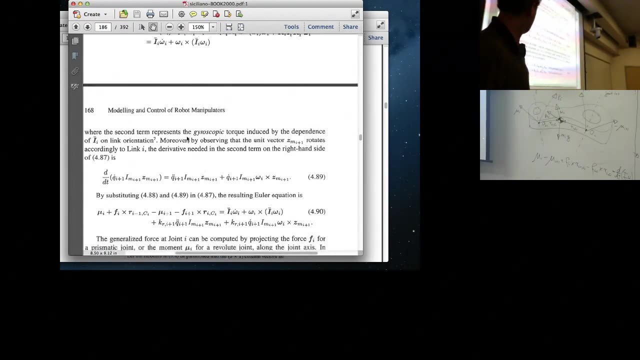 Putting a cross product operator instead, And blah, blah blah, Ending up exactly with this. So we get basically this formula on the right: I want the entire thing, The entire thing. So can you write it more nicely somewhere? The? 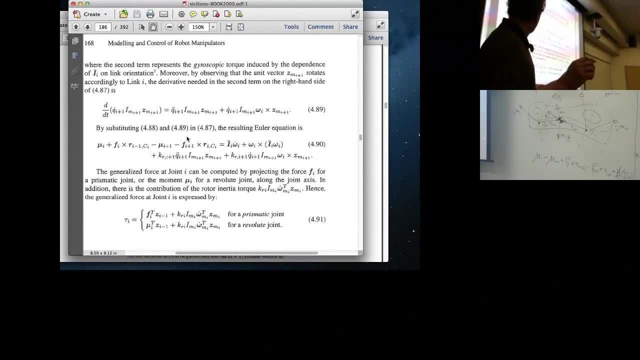 The, The, The, The, Yeah, Yeah, He has what I want. So the, This is all motor line, It's all from the motor. We can ignore that for the moment For our little derivation. So we have. 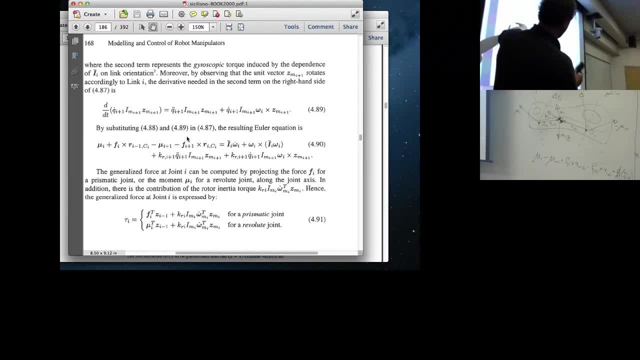 Momentum, Momentum, A momentum from the force on the left side. Momentum, force on the right side Equals basically the change of momentum which we get. That is essentially the Euler formula. oh, so much fun. now what's important about this stuff? see, if we look at a 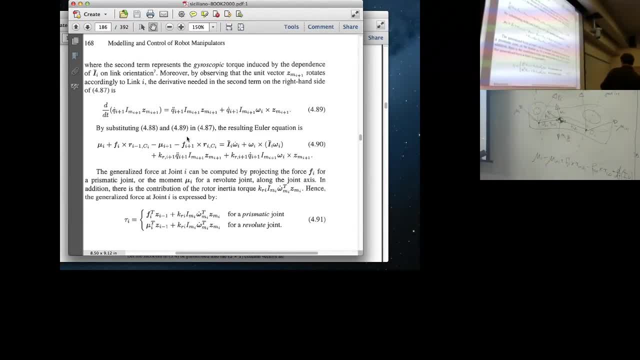 recursion it, you should be out the park. he wanted to express mu I as a function of it else. no, if I know from our previous force calculation that we've already done this is a kinematic thing. we know that mu I plus 1, we assume, is 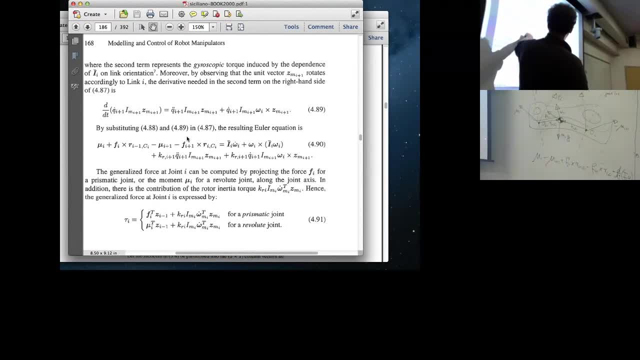 known from the previous link and at the very last one it's going to be 0 if when we know already from the previous link and all these, so we are fine. same idea of breaking a recursion. I know it's an a lot of. we create the. 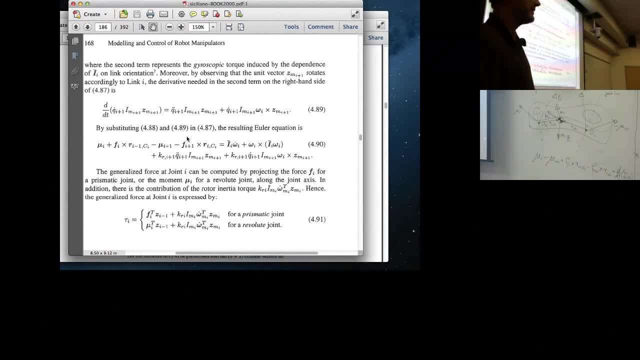 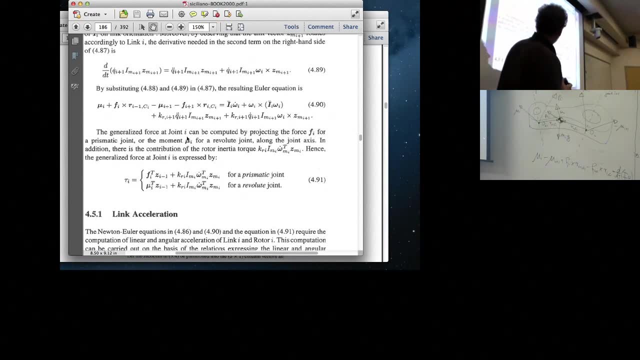 and not easy to pick up, but I think you get the picture at least. not not that I expect you to do right that fluidly or anything like this cool. and now we have that all. we just realized that there's occasionally some acceleration extinctions and I mentioned that to you before. so link accelerations we had. 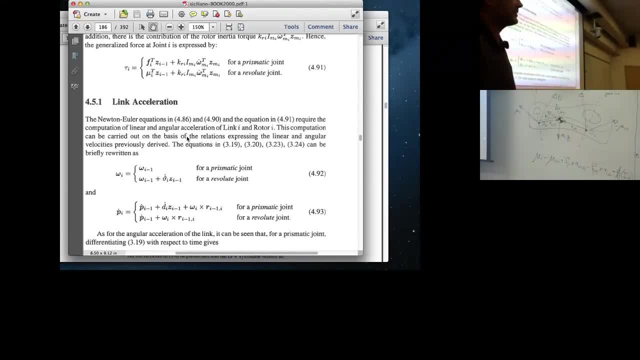 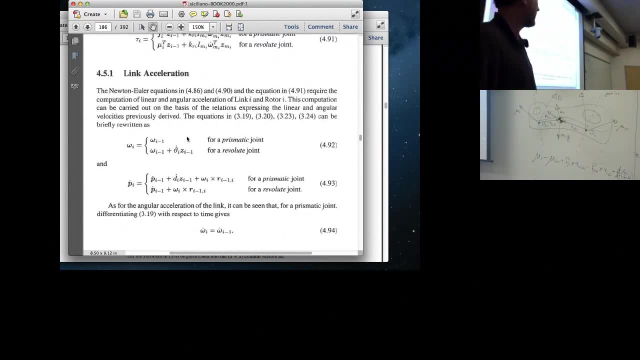 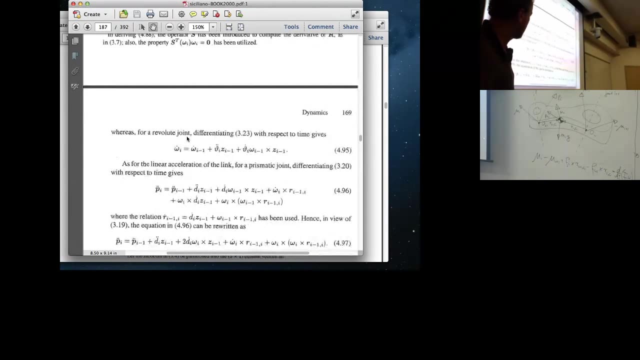 before these were the link velocities and now he does the entire mess for adding another point on this equation, another dot. I'm not going to go, it's just massive. I'm don't want to do this. it's just taking derivatives, doing again getting lots of cross product, figuring out what's good at that about? 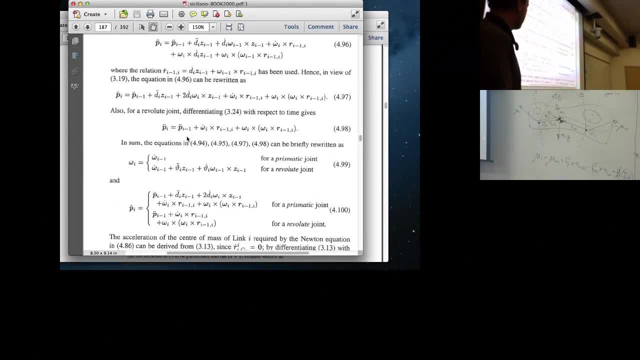 them and here's what I like in some you get basically equations for our prismatic and revolution. that is, the axle, the angular acceleration and the translatory acceleration acceleration. look like these things. okay, yeah, these are the if, the yes in the theta double dot, it's the acceleration of this particular degree of. 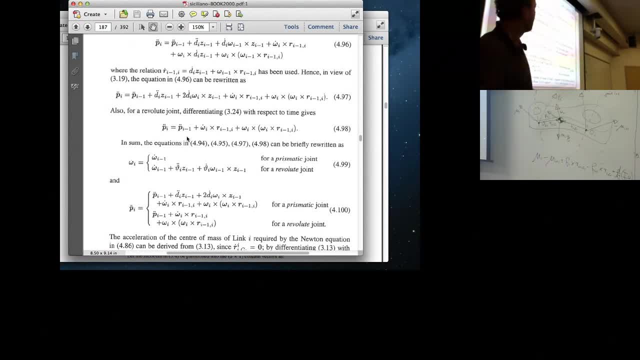 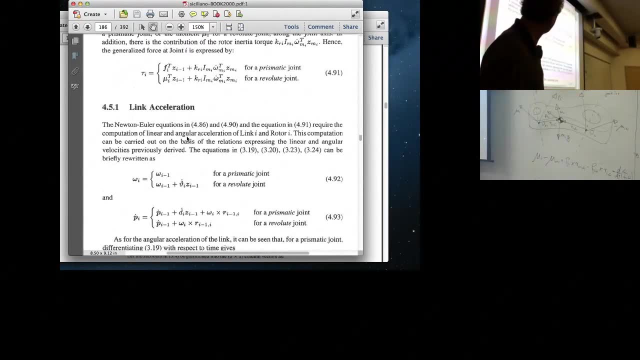 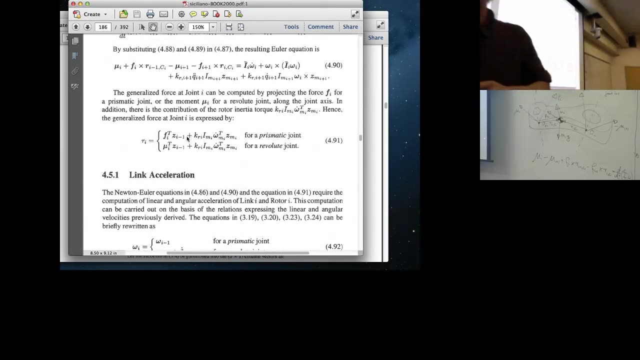 freedom. I did not mention one thing properly. I just go back for a second and you forgive me. what our, what the algorithm, Newton algorithm- does is telling you how to express a force on the left with respect to all the knowledge we have on the right. the same. 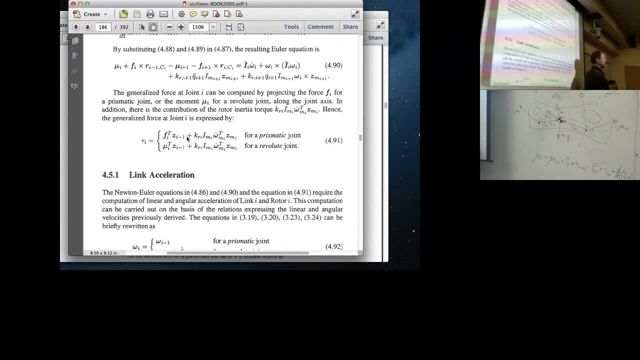 with the momentum if you want to know what's the torque and degree of freedom has to generate. like if I compute here at some point in you are. so how much does your motor have to support? how strongly does it have to control? how much does your motor have to support? how strongly does it have to? 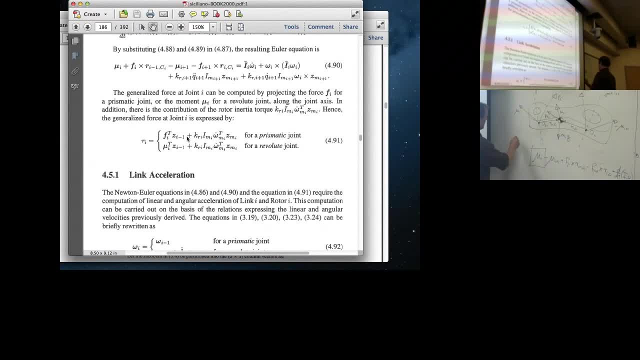 push. and that's very simple. you just take mu i. it's a vector, and you basically project it, the inner product, on your rotation axis or your axis of movement, which is di. that's the component the motor has to hold out. again, all the other components of mu i would be supported by the 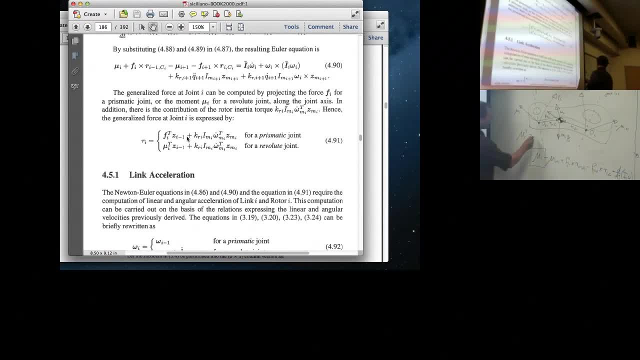 mechanical structure. this is how we actually get to the point that we get our tau i's. this is what he has basically gave it in here and I did not mention that properly. so mu I in a product with the IP, this motor stuff- forget about this- gives you four revolute, joins the. 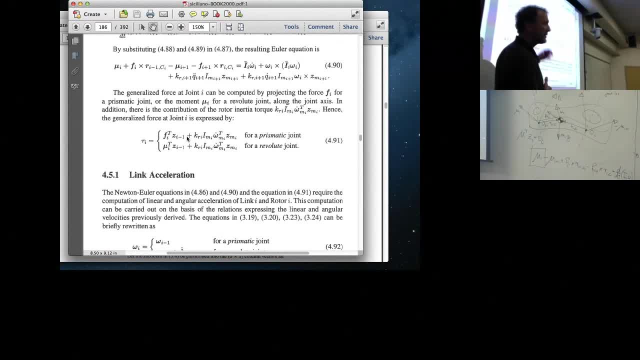 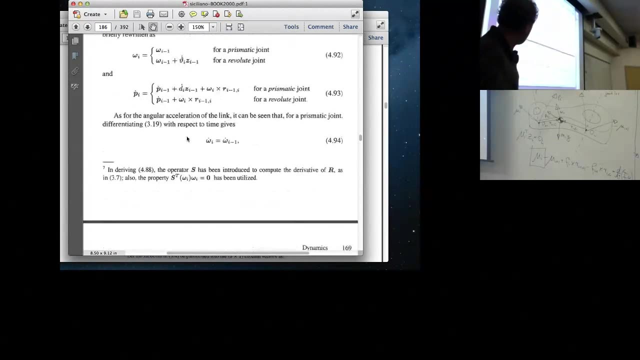 torque, and if it's a prismatic joint it's just F? I in a product, it with the eye. I should not have forgotten that, since that intention is the quantity which we in the end want when we do dynamics computation. so you're solidly happy. I see that I'm solidly tired and I think we try to go to the summary of. 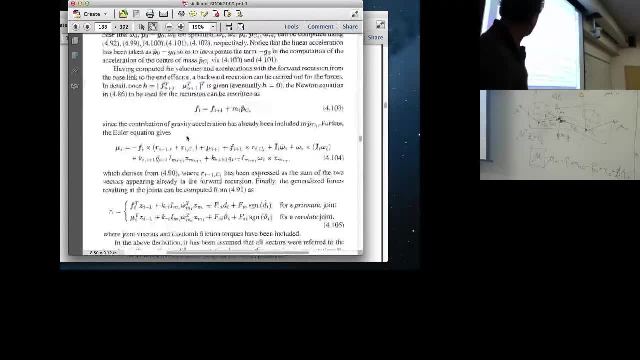 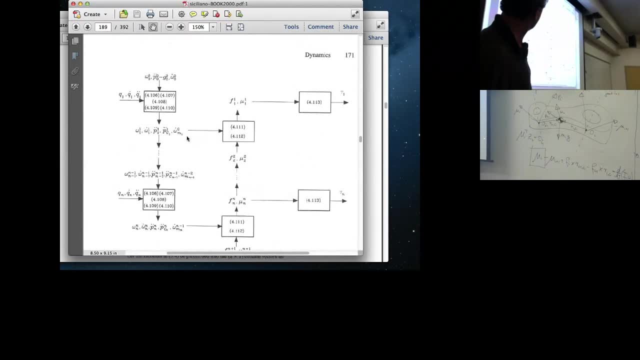 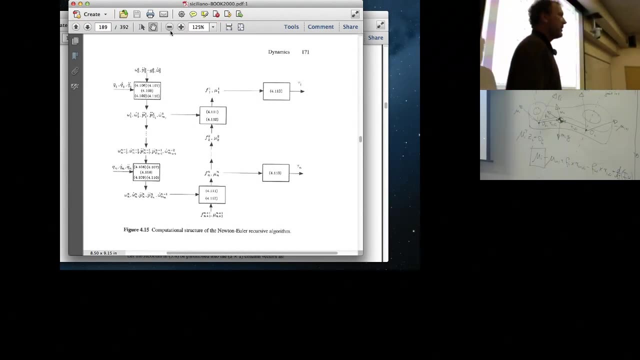 all of this. that's kind of useful. this is all yuck. there was a nice figure, there's still a nice figure, so let me make this a little bit smaller. and this figure is useful to just summarize what's going on. all the equations are somewhere, written somewhere, and he has been the equation numbers at various 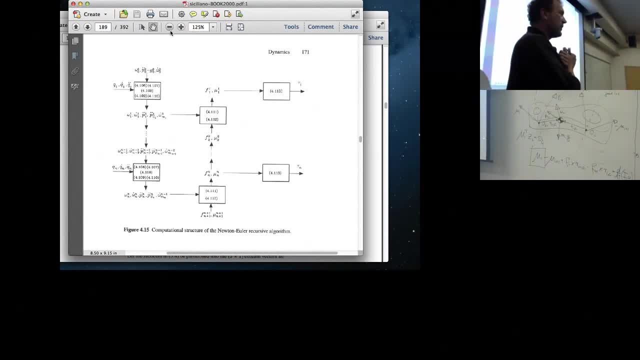 points. what do you have to do to compute Newton, Euler, so essentially they straightforward. get rid of this picture. we want to get to forces and torques at every degree of freedom, but what we need is velocities and accelerations at everything. so what we're going to do is: 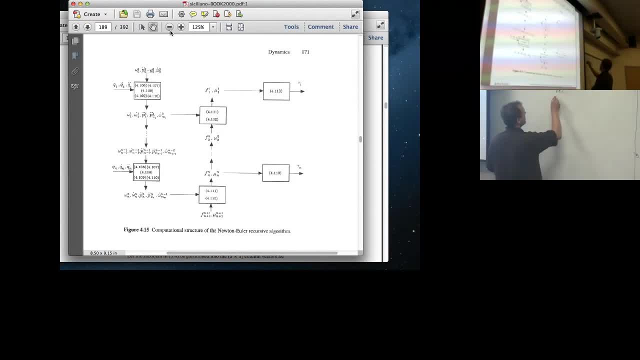 first we compute the force, and then we compute the force, and then we compute the velocity and accelerations at the first step. and how we do that? again, look at the robot. you actually saw that we can find recursive equations which compute velocities and accelerations and if you start at the base, the base has zero. 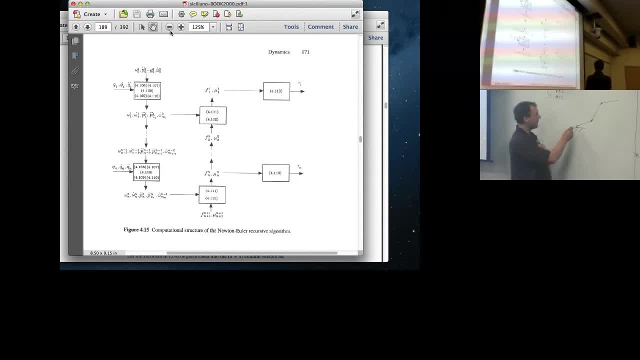 velocity and zero acceleration, so you can actually propagate from this knowledge velocities upward in the chain. that's basically what he tries to tell us how to integrate另外. hopefully, here we basically knowing our joint positions, velocities and accelerations, we can automatically compute the lot. joint angular velocities. 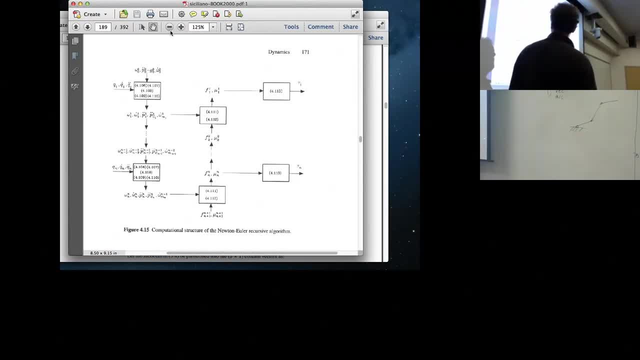 and translatory velocities and accelerations as well, for both quantities at every degree high up the chain. so there's a recursion which goes through this like this: this gives us velocities and accelerations and after we have this, that's the first concentration levels like this. so 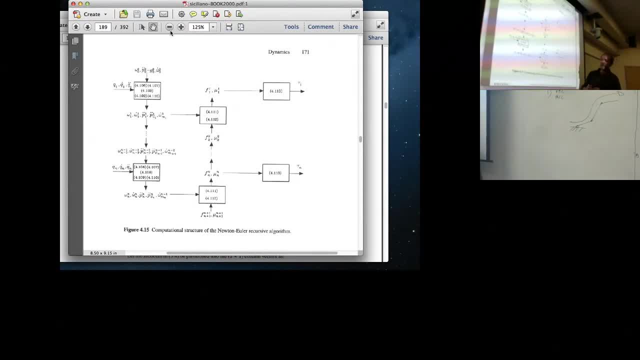 here to show you that the speed advantage of на очень large coefficient, quindi идти на this. we can actually now propagate back forces and momentum- You know there's no force and momentum at the very last joint- and basically go back the chain. 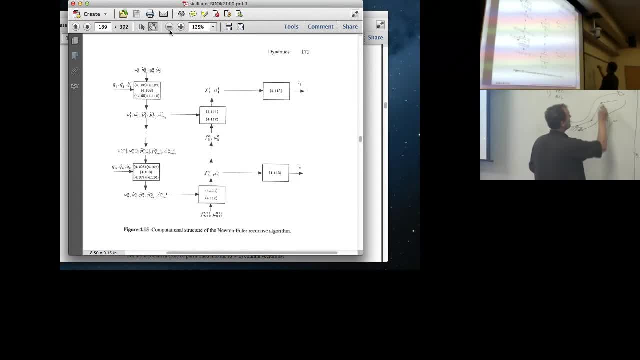 down there. This way we get force and momentum. and here we've got essentially all the- what do you call them? P, P-dot, P-double-dot, and omega and omega-dot. That's essentially what Newton-Euler does. You do a first path, get all the. 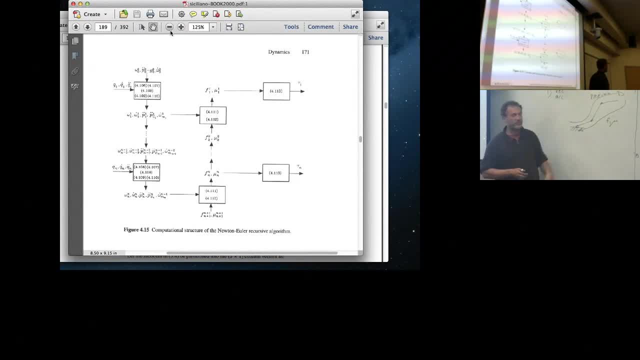 kinematic stuff computed. then you do a backwards path, you get all the forces and you projected every degree of freedom in the end, the force of the momentum vector in the axis you want, and you get the equations of motion which we want. 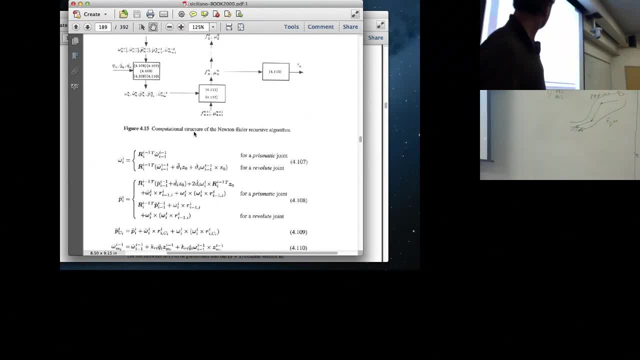 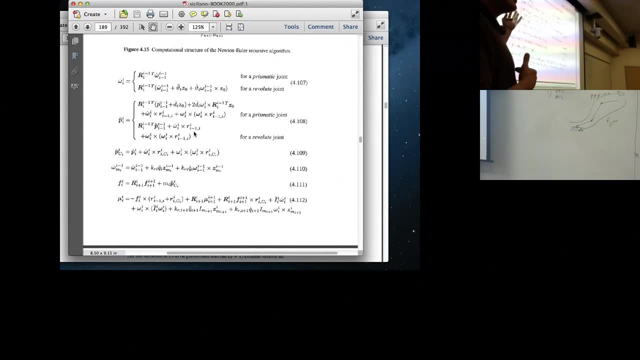 Oof, so beautiful. Here is all of it in one happy summary. I believe These are the occurrences you have to do In the end. it's not so terrible if you look at this. You just need to know all the quantities. skip all the motor components, get in. 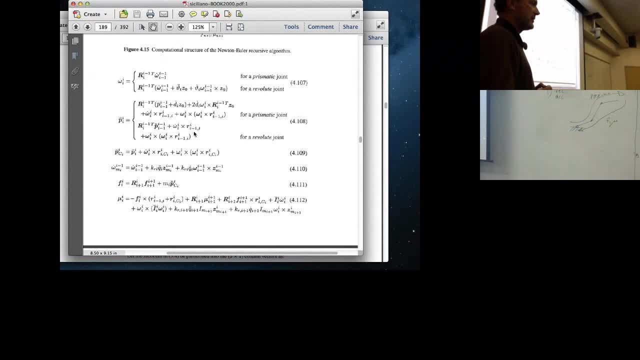 touch with the superscripts and subscripts and you're happy forever after. But now we're combining literally everything. We're combining our knowledge of kinematics, coordinate transformations and now a little bit of force So you can get all the forces and torques to get the entire dynamics of the. 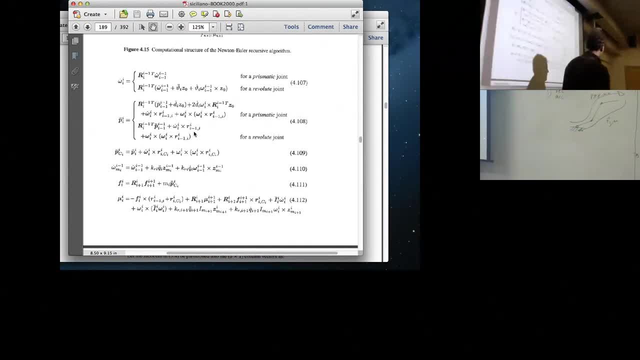 system model and that becomes just incredibly efficient. That's the beauty of how it works. I'll be doing it time-wise. Good, This is nothing new. So out of this equation, in the end we get our little trend, which I mentioned the last time. B of Q times Q. 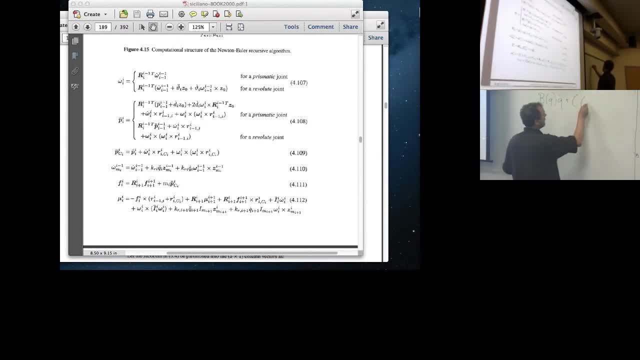 double dot plus C of Q, Q dot times, Q dot plus G of Q equals tau. So for every degree of freedom, basically, what does he input to any dynamics algorithm of this kind, which is essentially what's called an inverse dynamics algorithm, since you have to house the forces or torques on the 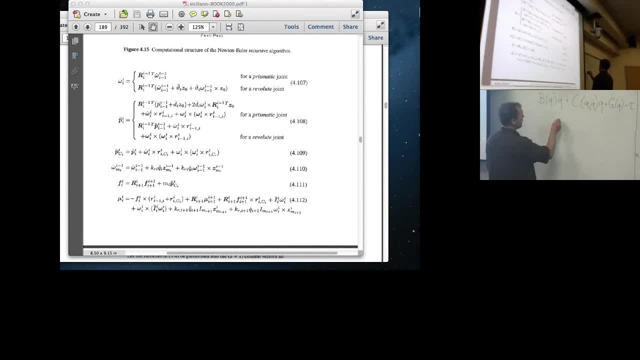 right side and all the other stuff on the inside. So if you know Q, Q dot and Q double dot, for every degree of freedom you have, you automatically create the forces or torques tau, and every degree of freedom you have You can compute them. 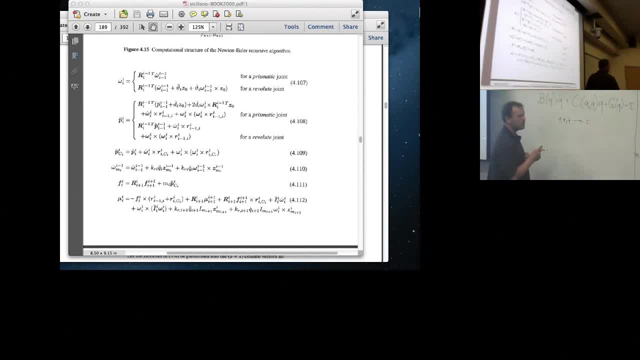 Which also means, if you think about it, let's assume what's the state of a two degree, of a second-order system. The second-order system is described by position and velocity. And assume you know that you want, from this state, accelerate in a particular way, make this Q double dot desired, then that would 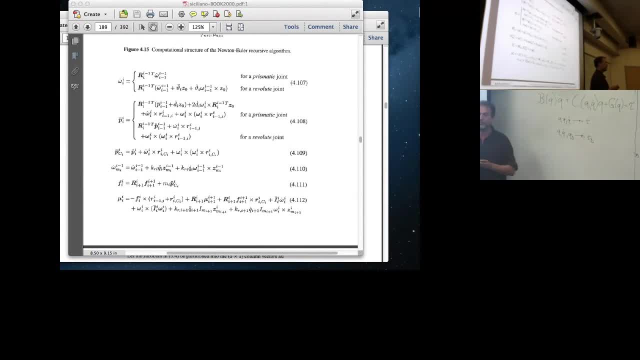 tell you what are the torques which you have to put into the system in order to achieve that effort. Now we're getting back to control. you have to put into the system in order to achieve that effort. Now we're getting back to control. 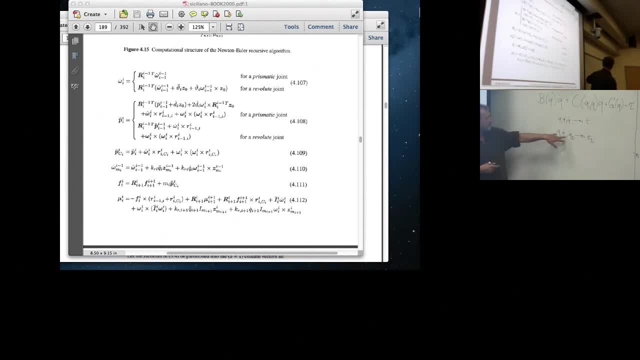 This is what we're going to do primarily the next time. So, knowing these functions, here we can compute torques which accomplish a particular state or which take us out of a given state with a particular acceleration. This is all we're going to do in robotics in the end. 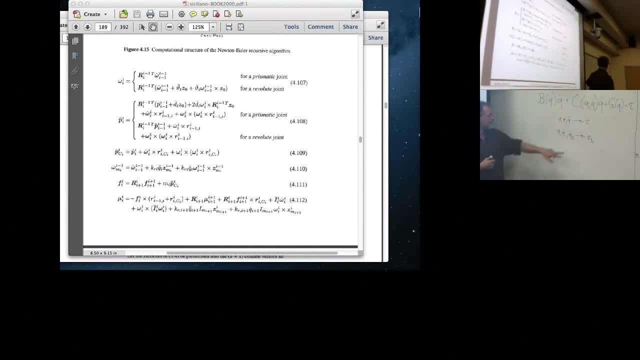 Basically plan some position, velocities and accelerations and try to figure out what torques are the right ones to push us in this direction and accurately as possible. Now as a remark, there's kind of a big difference between deriving this here and then writing an equation like that. It took people a while to figure out that the equations can. 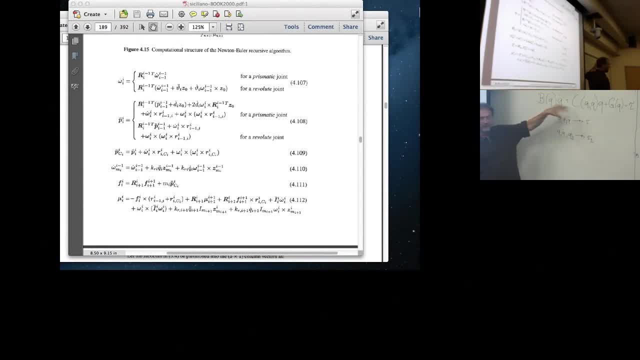 be written like that. It was not so straightforward. But after you realize that what you now get- if you have someone who can write this math, it's just a function. okay, You just create an inverse dynamics function. Oops, cannot write anymore. Let's call it. 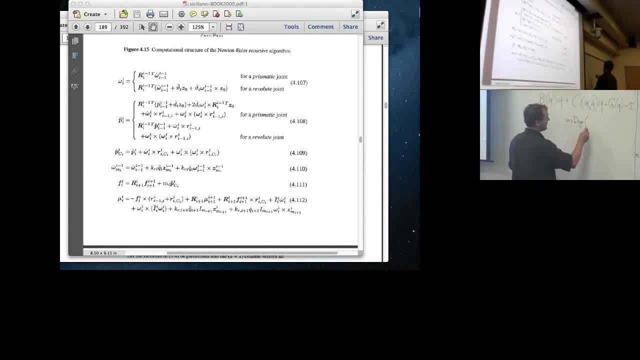 inverse dynamics And just in some pseudo coding. this is a vector q, vector q dot, and vector q double dot Outputs a tau. These are all vector coordinates. That's the C function of Java or whatever model function you would like to have. 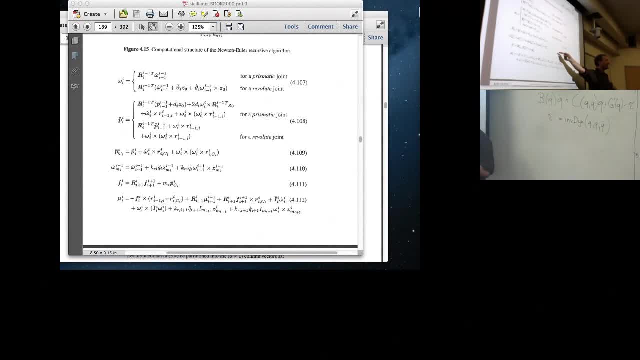 This is the stuff which is inside of that, So there has to be additional knowledge about the kinematics of the robot and masses and all these kind of things in relation. But this is how this thing in the end works. What is interesting about this now is if you actually wanted to get individual 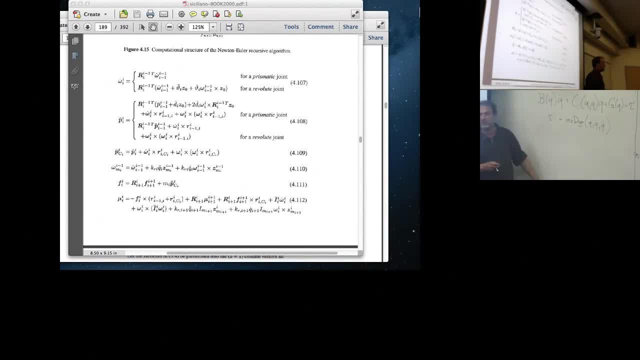 quantities of this equation. you can actually use that little function to help you. So, for instance, if you just wanted to know the gravity component, how much gravity force and torque do you need to support the robot when it's standing still? Well, very simple to say: the tf to zero and this to zero, one year level function, and you know that. 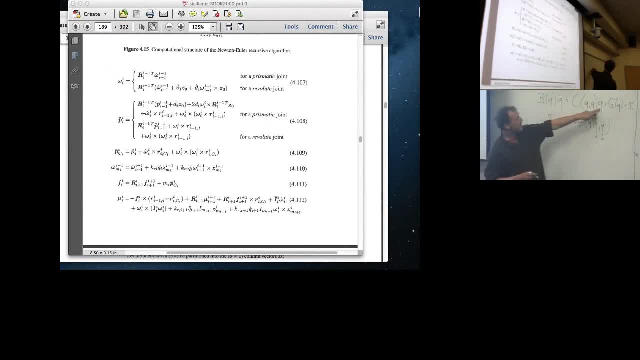 if you have q double dot zero, this will be canceled. If you have q dot zero, this will be canceled. so then you give only the gravity forces to the torus. It's a nice little function to use And you can play other games If you just want to know what's the contribution from the 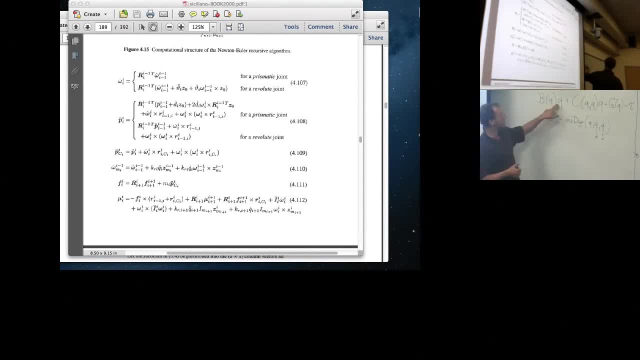 Coriolis forces and Contributors forces. So if you take q double dots to zero, you get rid of that. You compute g of q, as I just told you, and then you compute basically- Sorry, wrong sequence- You compute g of q first. You know how to do this. 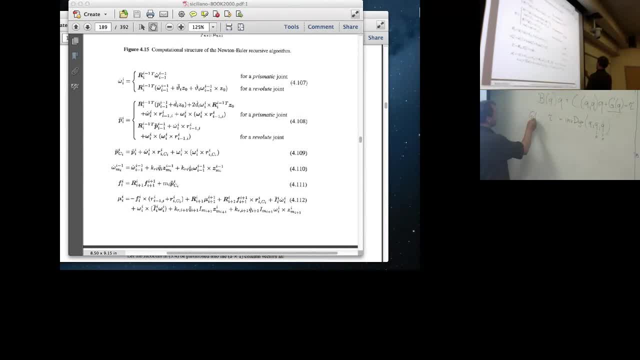 This was here And so this here basically was g of q. Then you said: basically you just compute c plus g and this basically you do, tau equals inverse dynamics of q and q dot, and this here is zero, and then you can subtract the g from this and you get the c term. So we can basically mess.